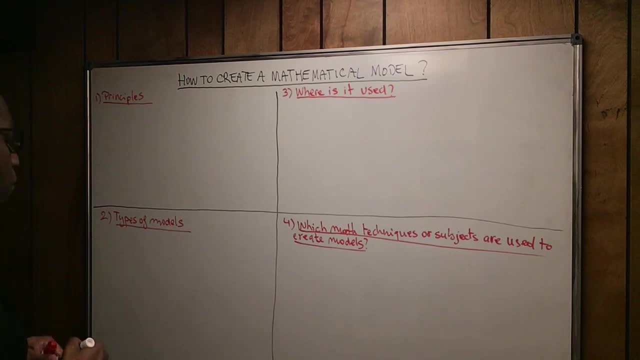 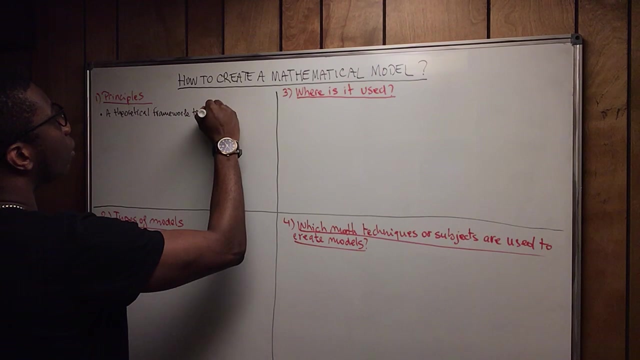 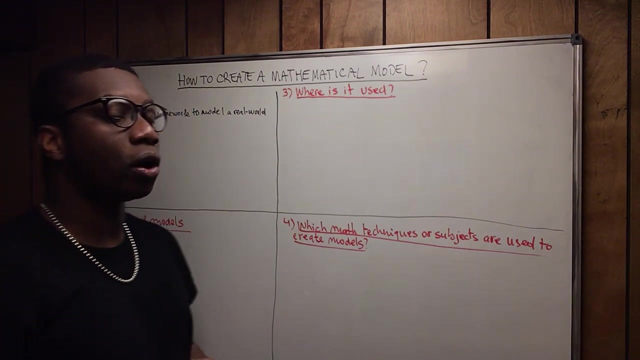 what is a mathematical model? So a mathematical model is simply a theoretical framework to model a real-world scenario. Okay, So a mathematical model is in fact a simplification, all right, of a real-world scenario. So you are basically trying to explain a real-world. 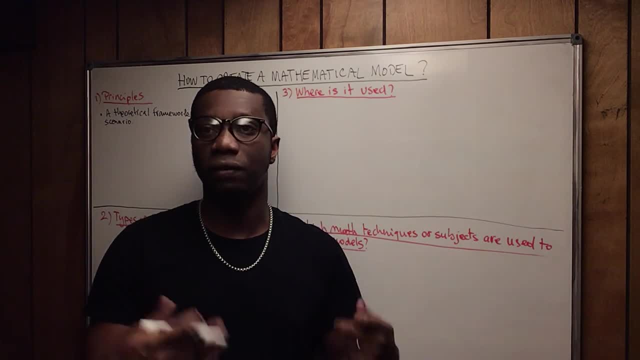 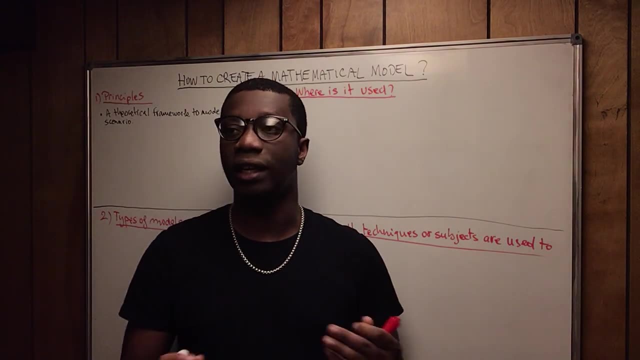 phenomenon. That's why we use we start developing mathematical models. It's for us to have an understanding of what's going on. So we start developing a mathematical model. It's for us to have an understanding of what's going on. Of course, a mathematical model cannot take everything into account. It is 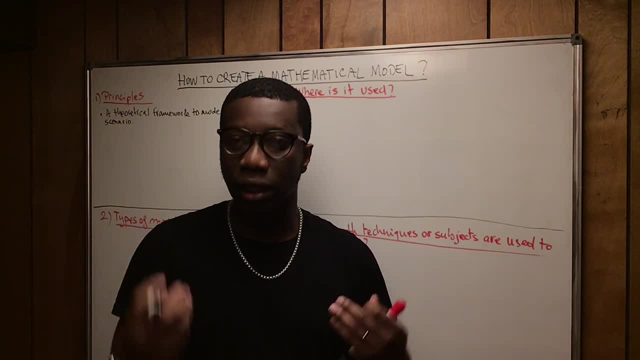 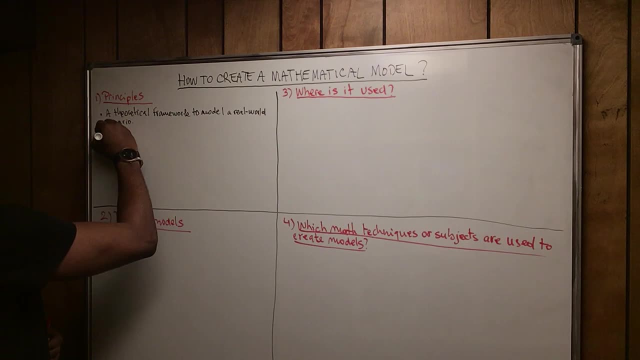 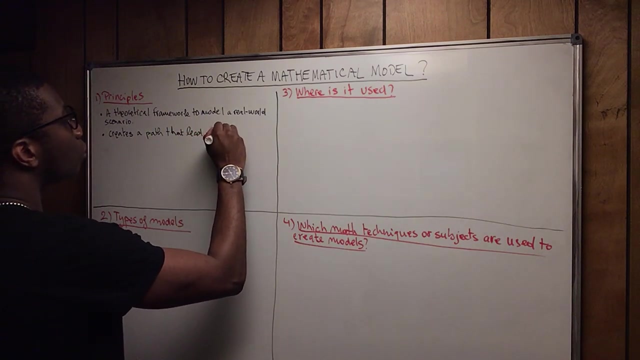 impossible. That's why the skeleton of the model is a simplification of it. All right, And then why do we create this? Why do we create a mathematical model? So the purpose is that it creates a path that leads us to the testability. 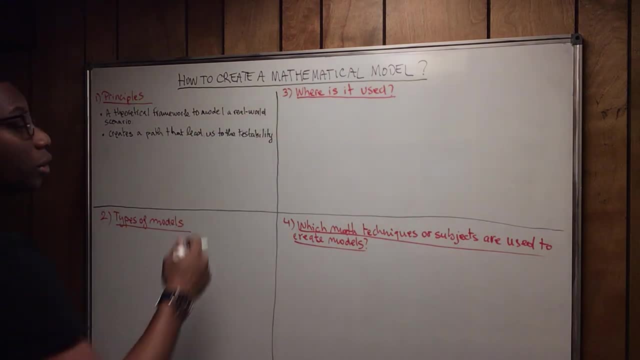 I don't know if the accessibility is necessarily the right word, but I use the word testability anyway. So it leads us to the testability of the model. So we don't create the model for fun. we create it so that we can. 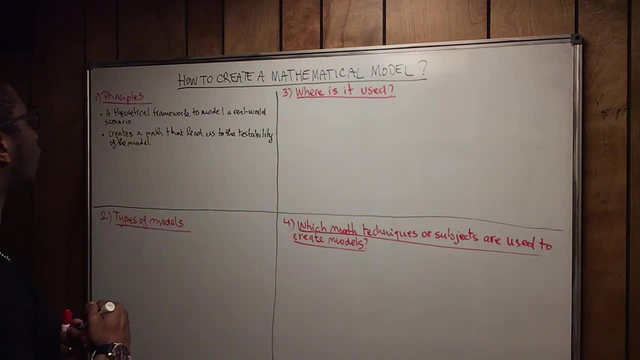 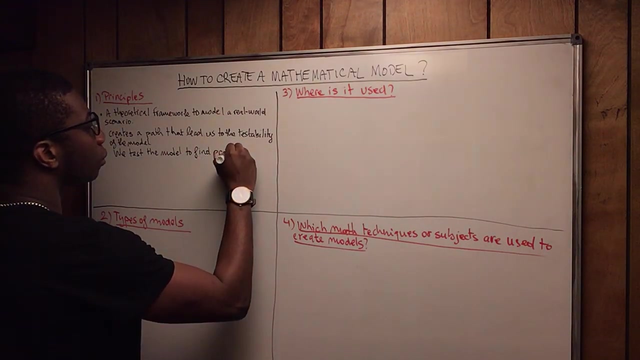 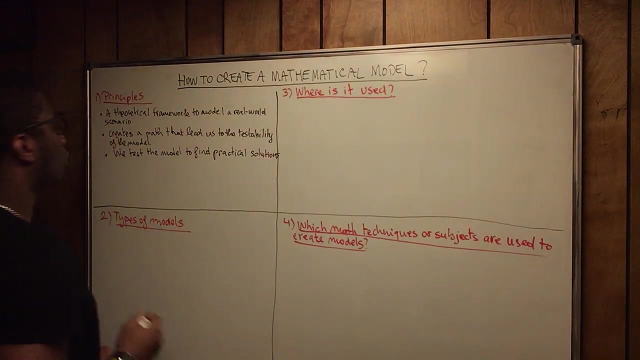 a way to test it right, and why do we try to test it? we test the model to find practical solutions. okay, so we test the model to find practical solutions. and what? what are the other benefits of a mathematical model? so he help us, helps us clarify our 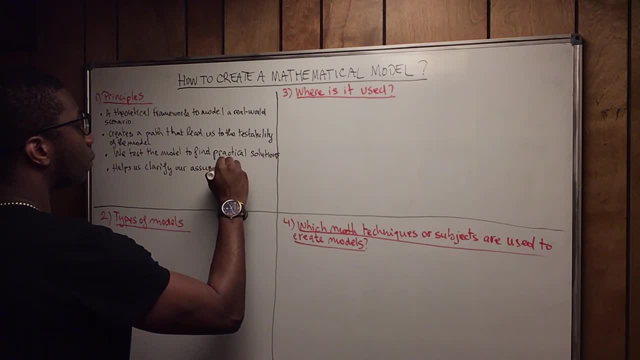 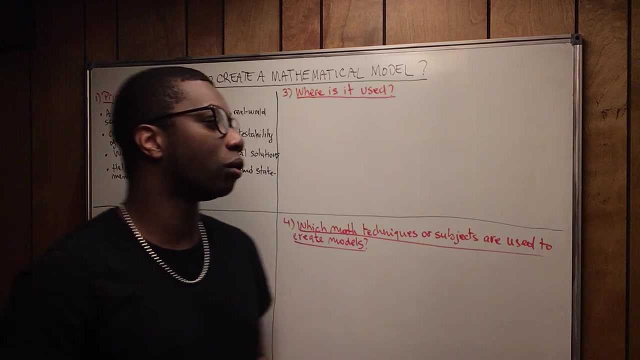 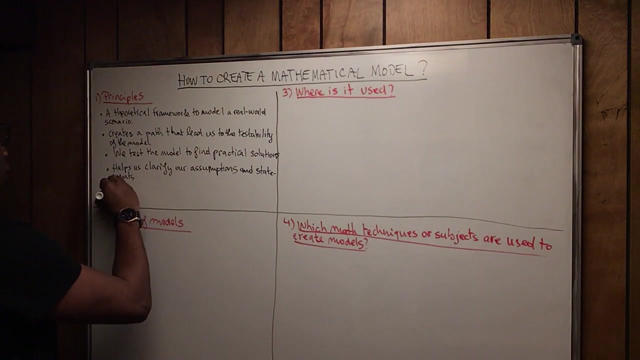 assumptions and statements. so when you create a mathematical model right, the purpose also is that you first develop your set of information using a priori, the a priori method- let me put it here- a priori method. so all your assumptions are a prior right. so you're describing a 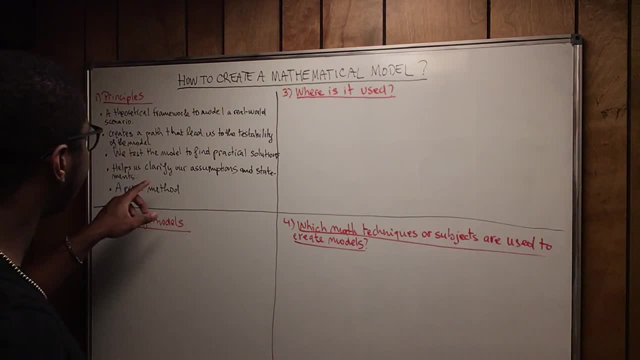 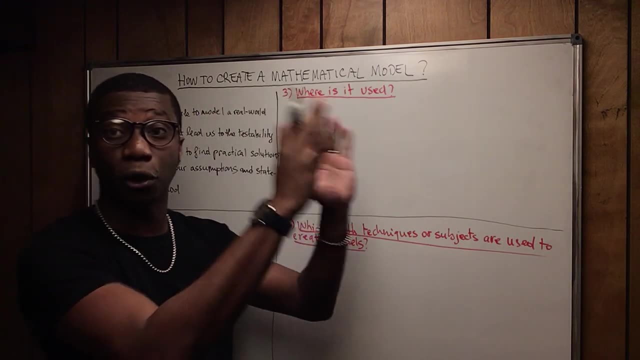 scenario. so it has to be a prayer right. and then you now use, you now develop the mathematical model in order to clarify if what you've developed verbally holds, because when you develop it theory verbally you can get lost in the process. it doesn't mean that you will necessarily. 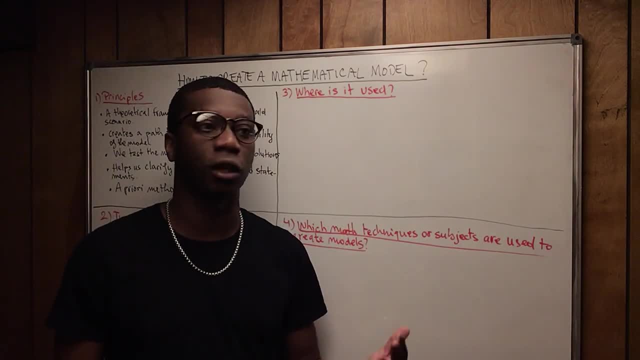 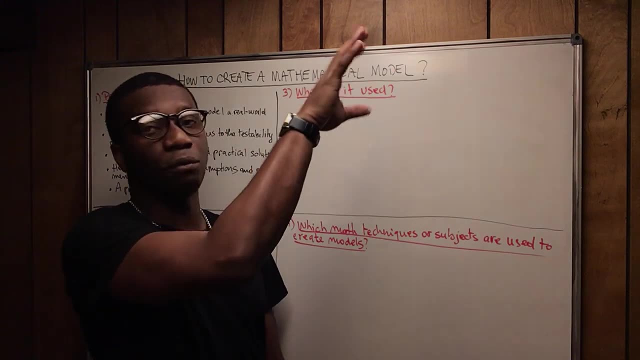 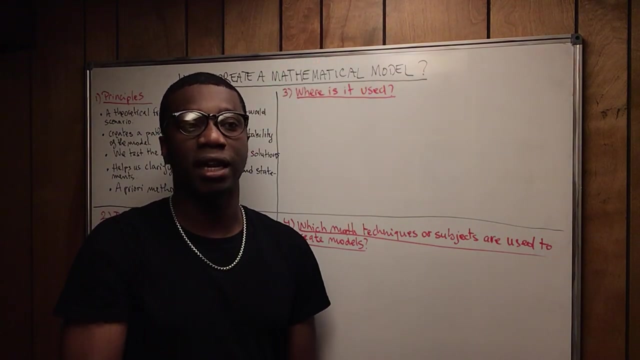 411 00Ч loss. of course not, but you could. so you use mathematics as a rhetorical device to see if everything you said in the a priori information holds in the math, in the mathematics. so all the big variables, so everything you stated that a part of. 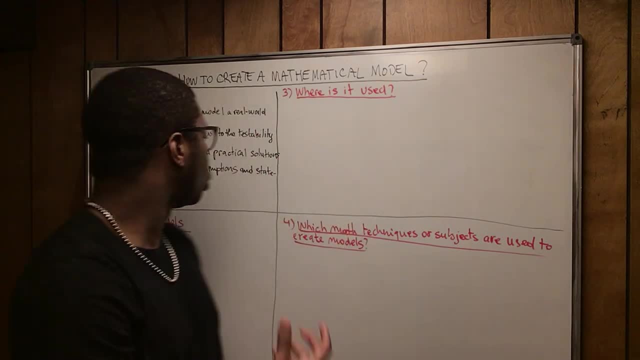 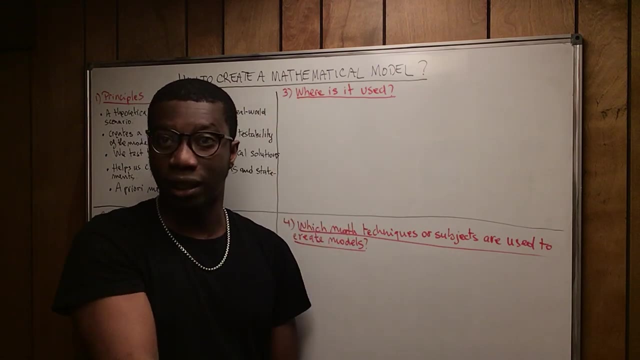 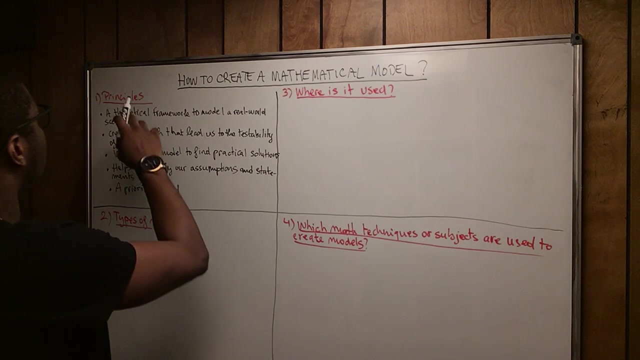 what you're going to be tested are the variables. so you want to make sure that all the variables you mentioned in in the a priori part are also represented in the mathematical model. so these are some of the principles of, or should I say the basic principles of, mathematical modeling, and now the next is the types. 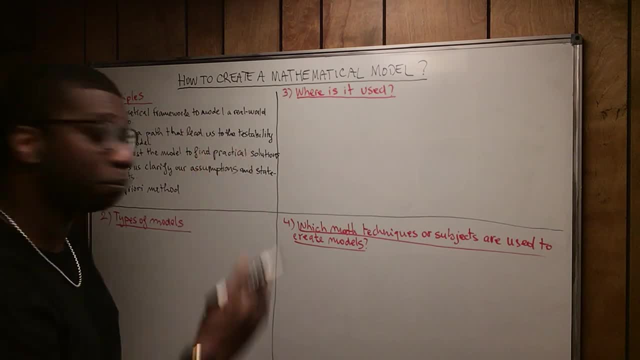 of models. so what are the types? in fact, the four types. you first have dynamic systems. dynamic system is one kind of mathematical model. I personally don't know how to use them is something have to work on. you have statistical model. this is what I do for living, so that I 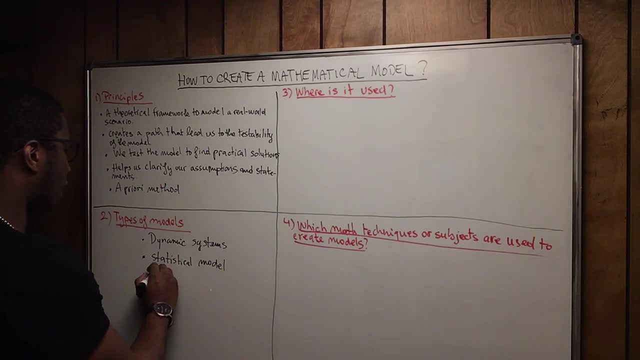 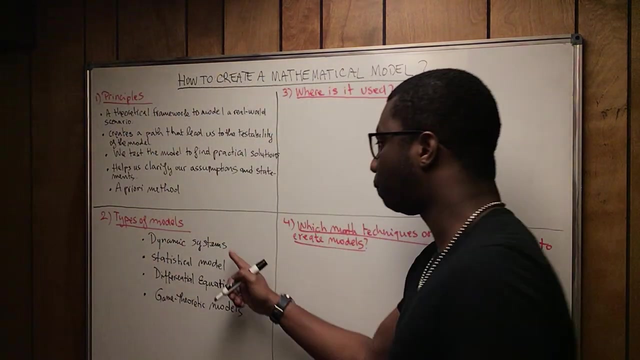 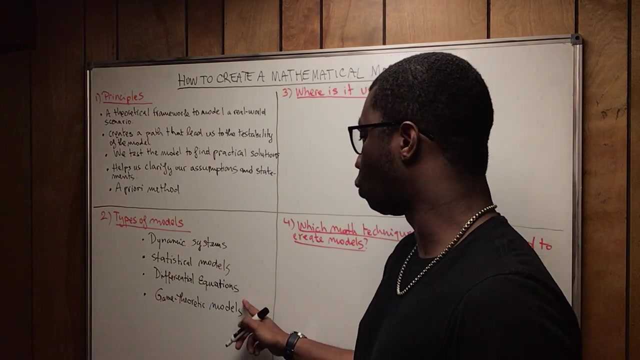 know pretty much I use that we gonna metrics all the time. then you have differential equations- okay, and then you have game theoretic models- all right. so you have dynamic systems, statistical models, differential equations and game theoretic models. so what i know for sure are these two. 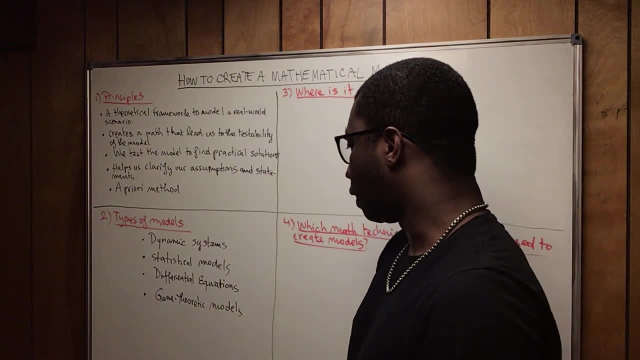 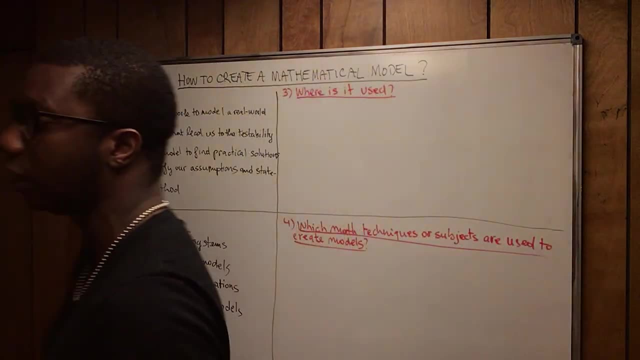 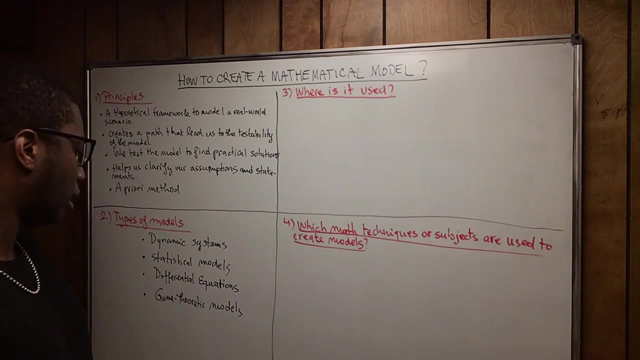 statistical models and differential equations game. theoretic i don't, i'm not too um keen on that yet, but it is used extensively in public choice theory, uh, which is the school of thought that um, i'm in in economics. so now the question is: where are mathematical models used, in fact? 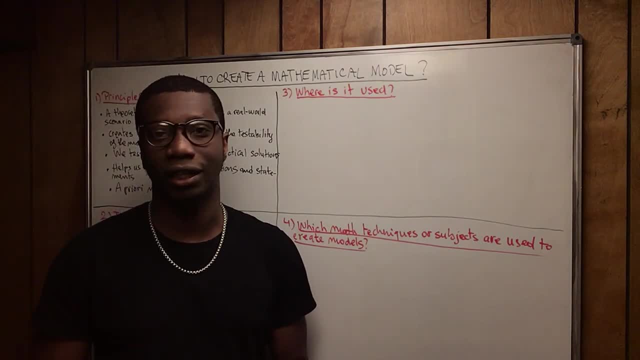 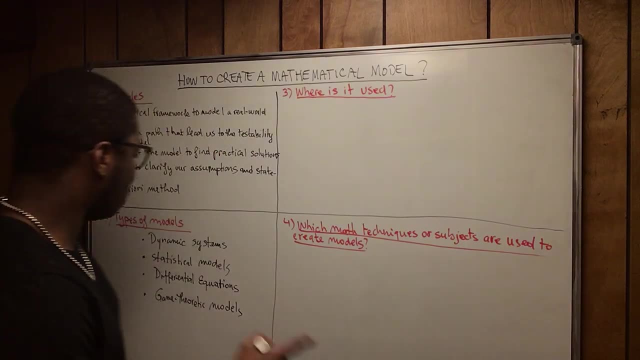 they're used everywhere, even in the water that you drink. it's based on a mathematical model, because the process of cleaning water is based on any of these models used they can use. so like, let's say, the pipeline company can use dynamic systems to develop the process, or they can. 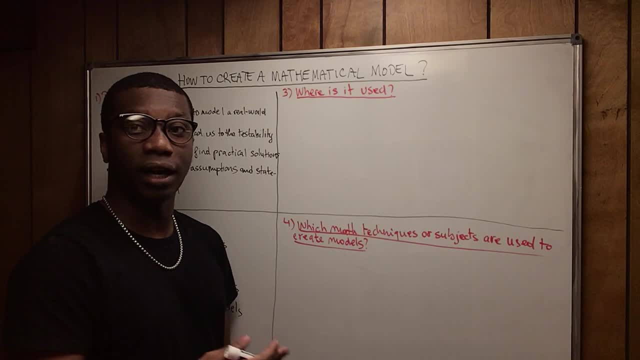 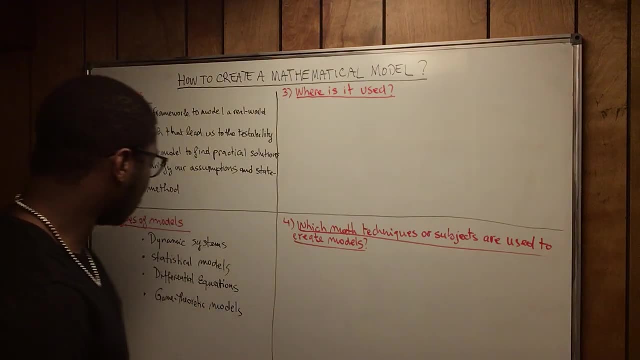 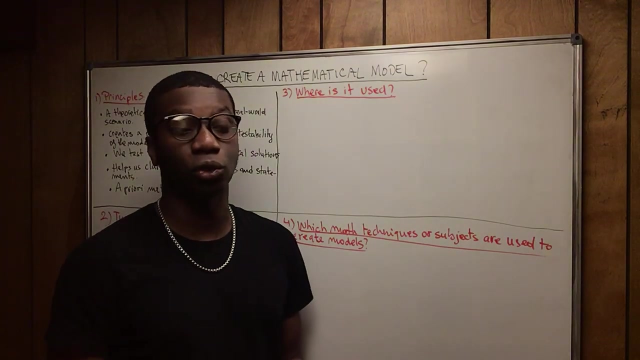 even use statistical models if there is the data. right, if there is a data, they can use that data to see the historical trend and then predict or explain. or they can use differential equations to also develop the process of cleaning water. so this is how far it goes, like it is used pretty much everywhere. so here, 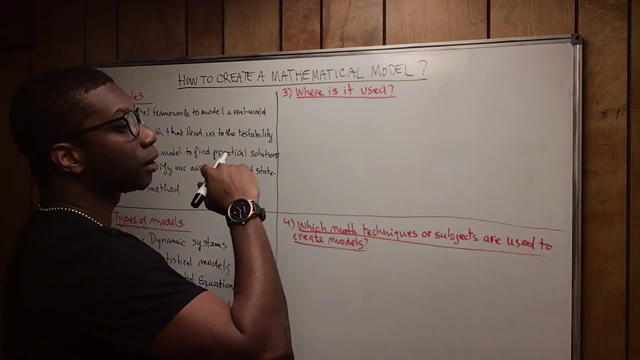 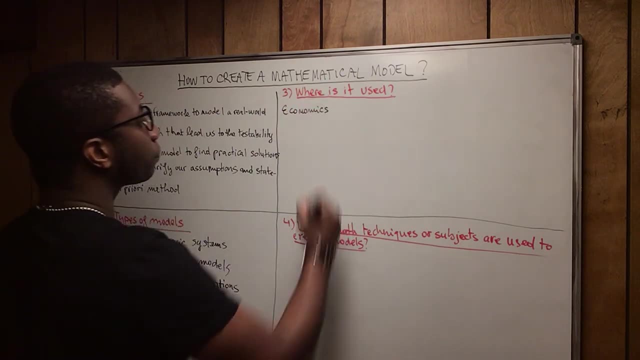 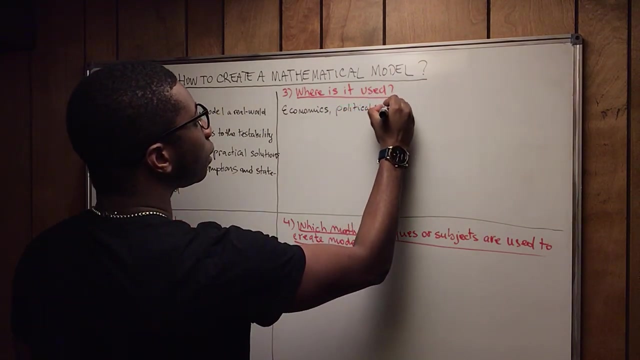 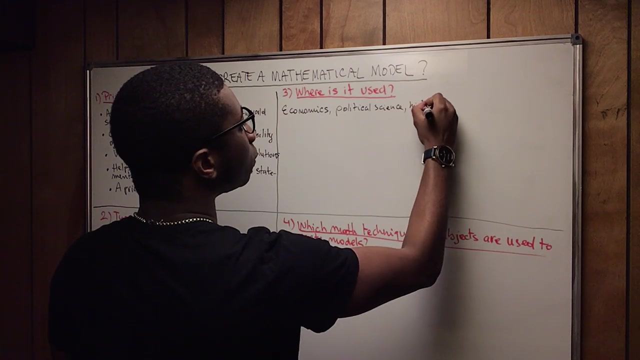 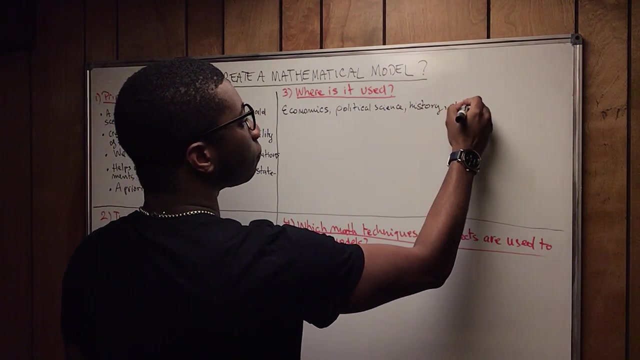 what I'm going to show you are the are basically the field of study. so of course it is used in economics. I start with econ, because that's what I'm in. it is used in political science- okay, it is used in history through plyometrics. it is used in physics, of course it is used in. 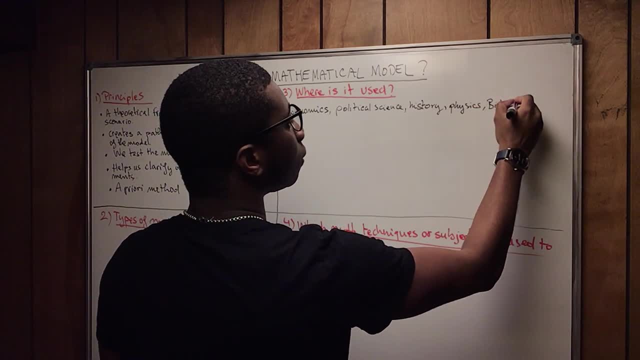 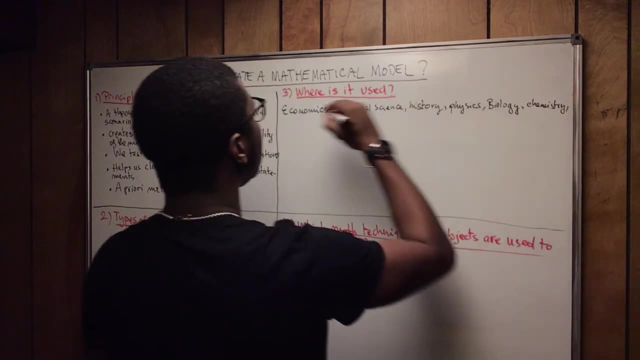 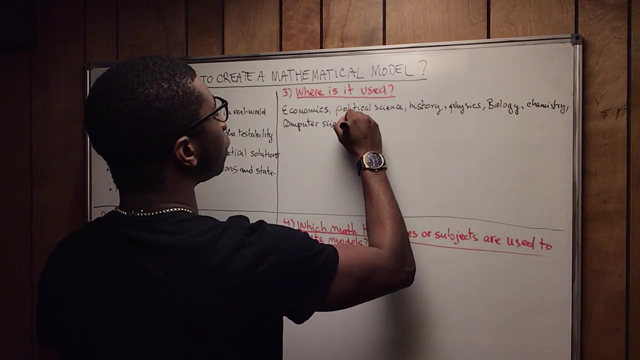 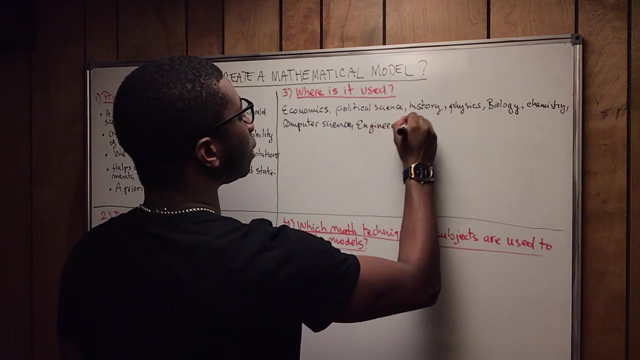 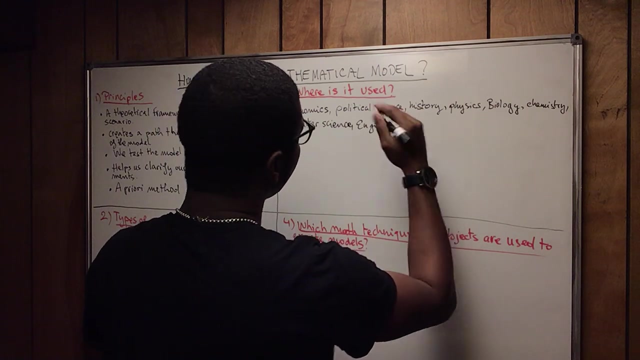 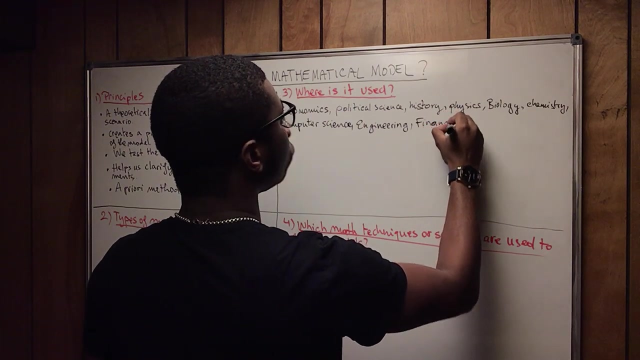 the biology. it is used in chemistry. it is used in computer science, specifically through discrete mathematics is using computer science. it is used in engineering- okay, whether it's mechanical engineering, civil engineering, biomedical engineering, electrical engineering, all kind of engineering you want. it is used in finance. a lot people use mathematical models all the time to make billions in. 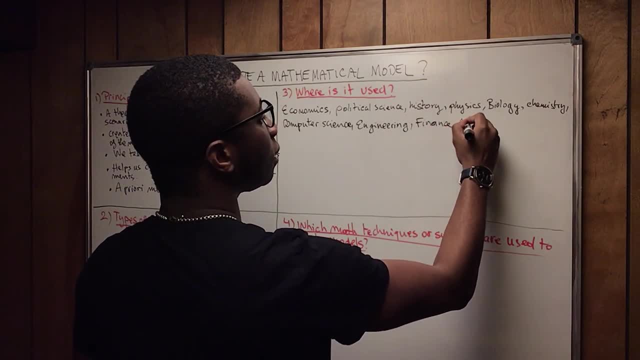 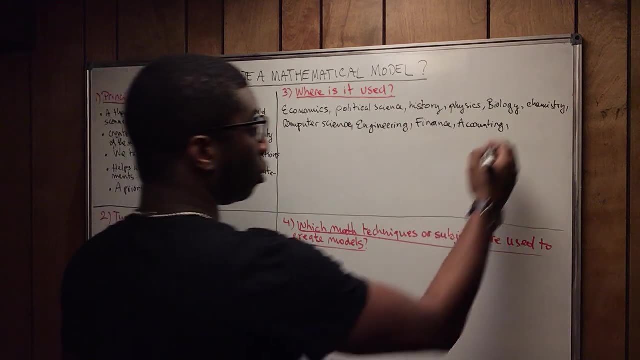 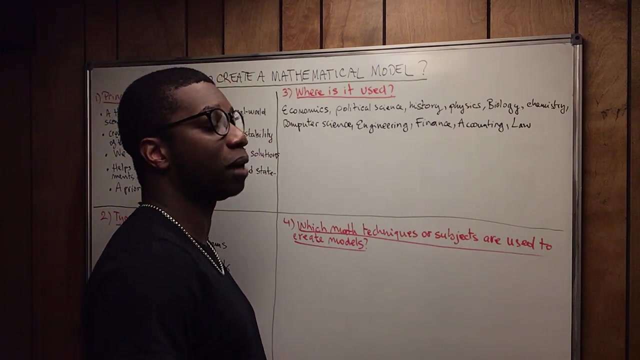 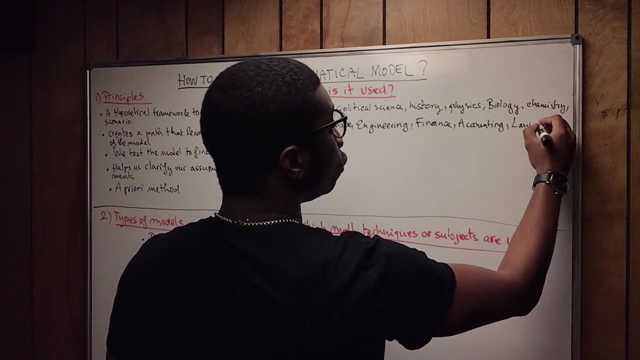 finance. it is used in accounting. that's what they use to develop new tax code. it is used in law: yep, in law, in law. you may say how you use mathematical models in law. while you use mathematical models in law to determine jury behavior, alright, so you use that. it is used in music: yep, even in music, specifically in music. 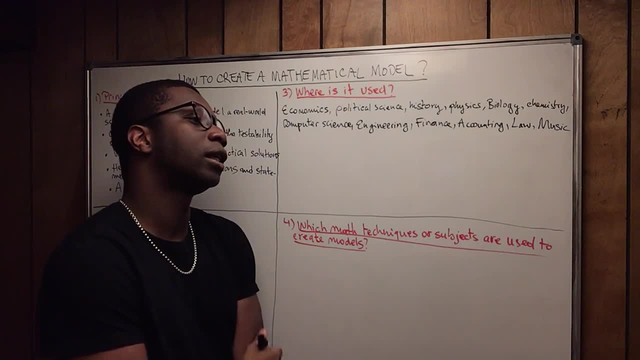 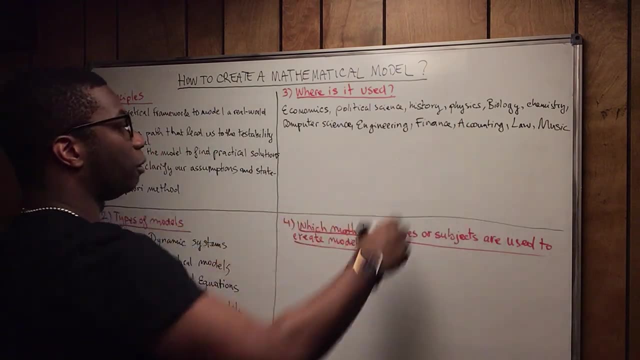 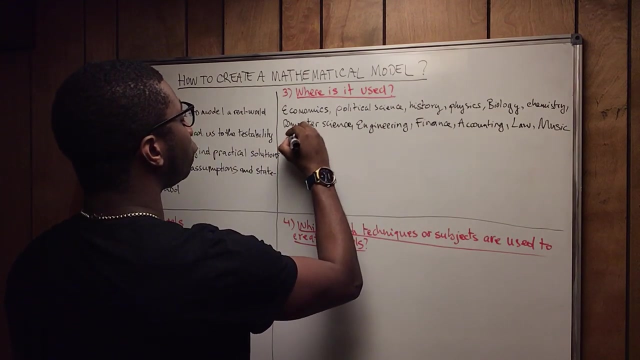 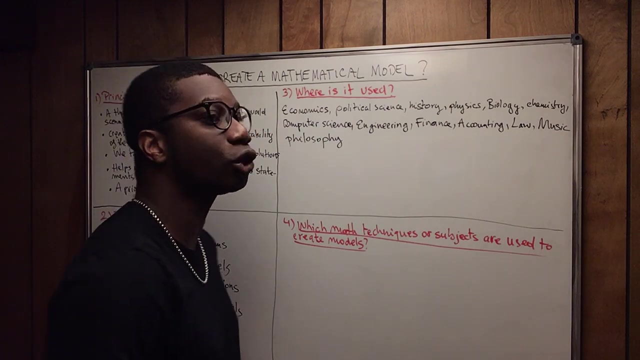 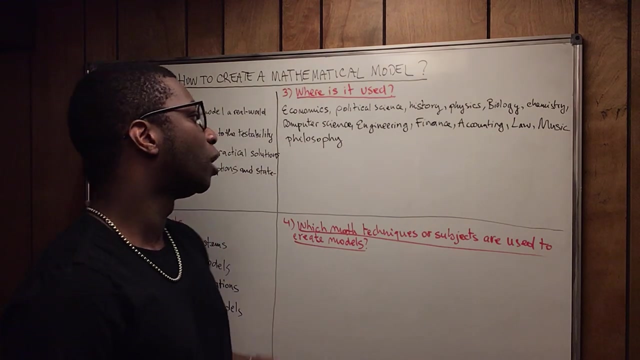 theory, you use mathematical models to determine the pattern of musical notes or even like sounds. so you- basically people will use differential equations for that. it is also used in. it is used in philosophy, so there is a branch of philosophy called analytical philosophy. so so for people who read a lot of philosophy, Robert Nozick and Bertrand Russell were to 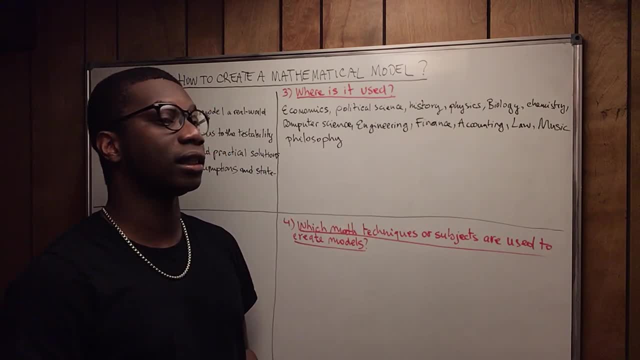 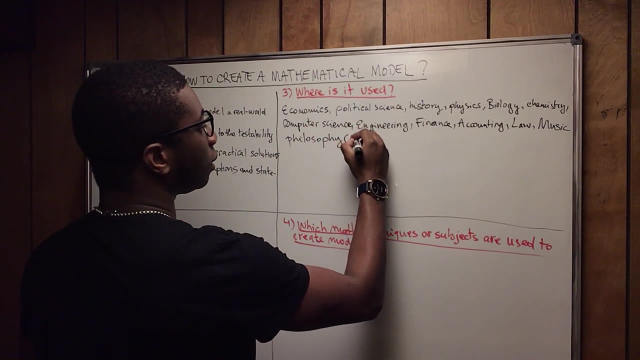 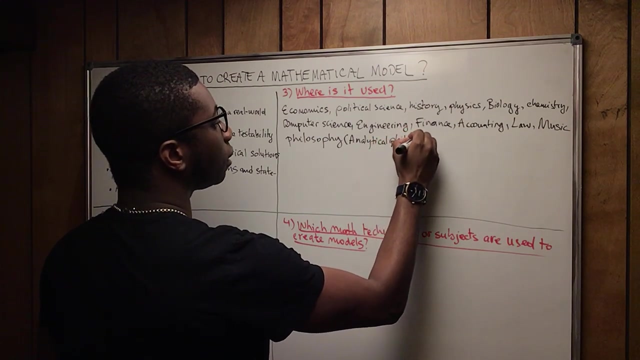 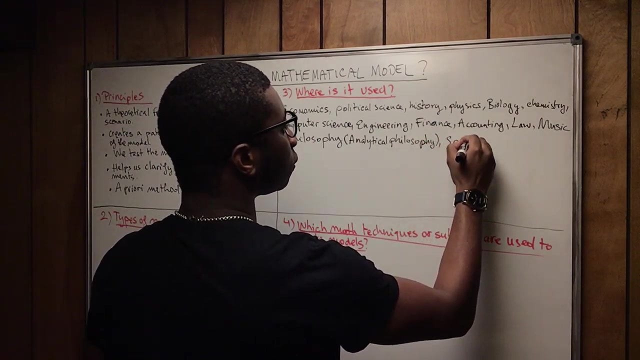 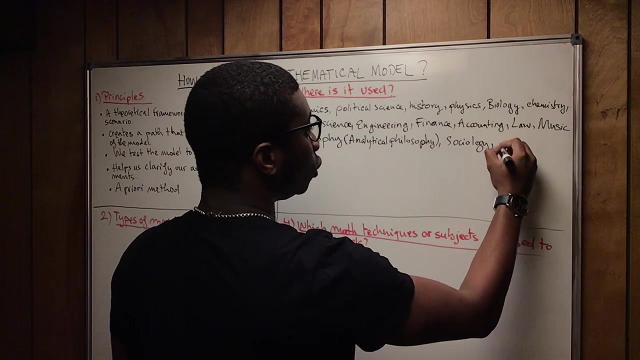 analytical philosophers, so they use math to in fact develop their philosophical doctrines. so you have- so let me put it here- analytical philosophy right, so it is using analytical philosophy. it is used in sociology a lot. there's a branch called mathematical sociology and it is used in psychology and there's also a branch called 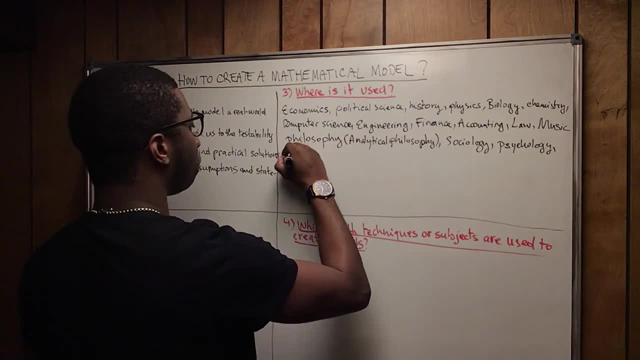 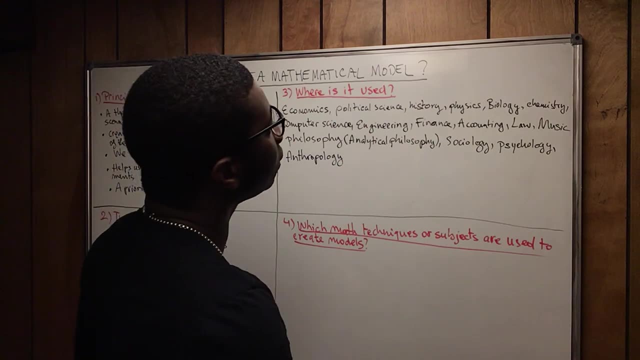 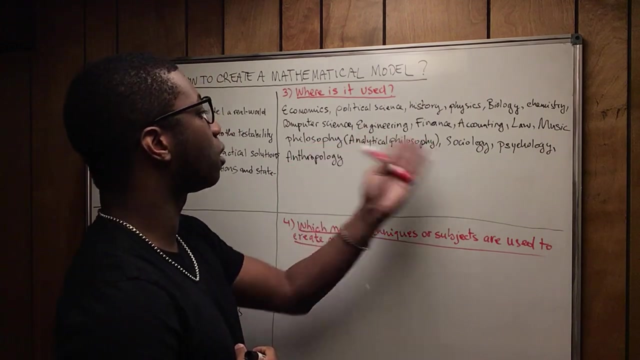 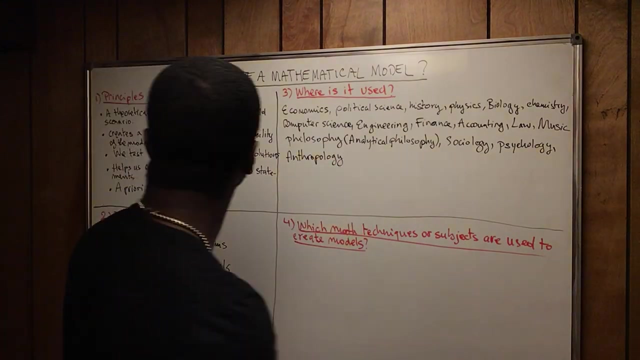 mathematical psychology. it is used in anthropology. I don't know if I'm missing any other field of study, but these are the field of study that comes to mind and mathematical models are used in any of these, any of these fields of study. so it is amazing. it is amazing. 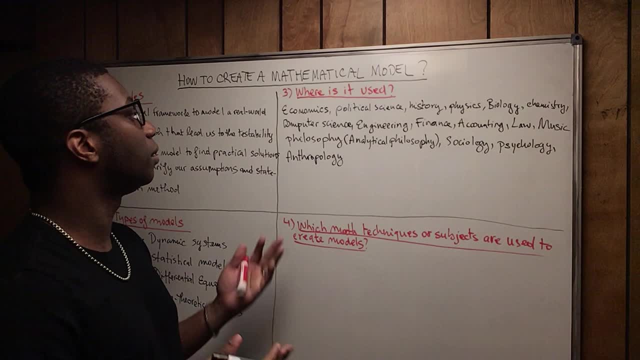 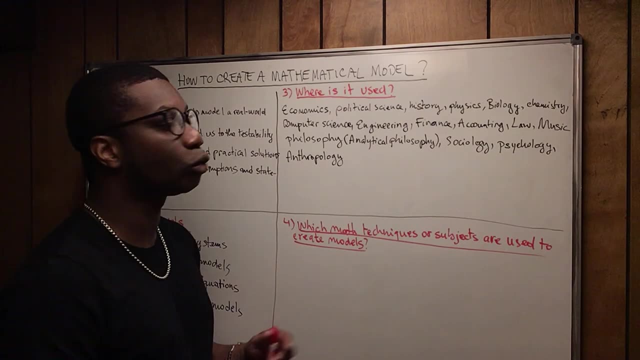 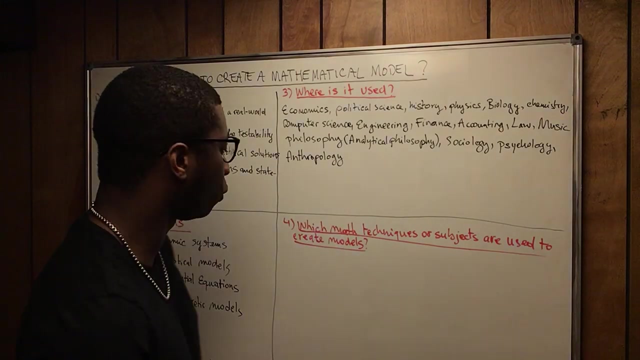 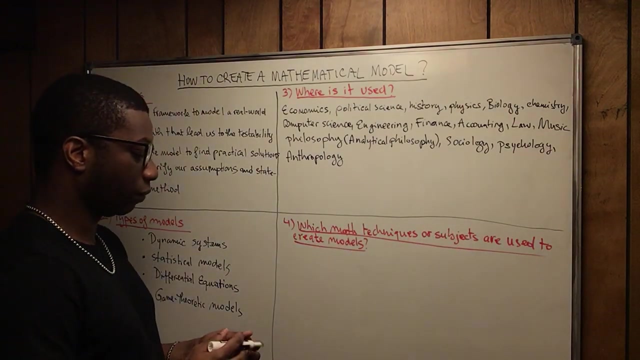 what you can do with math. yeah, it's a. everything we do, everything we use, are based on mathematical models. that's why I've been insisting on people learning how to use mathematical models. it's very important now which math techniques for subjects are used to create models, so you 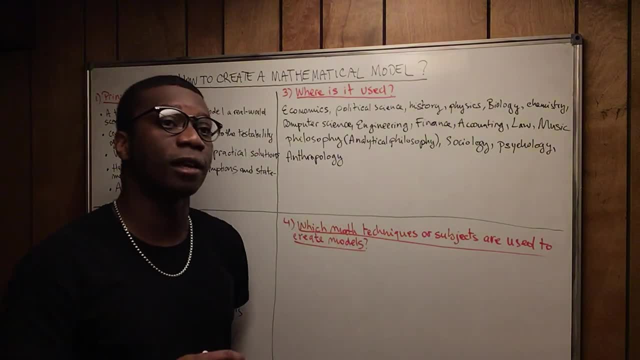 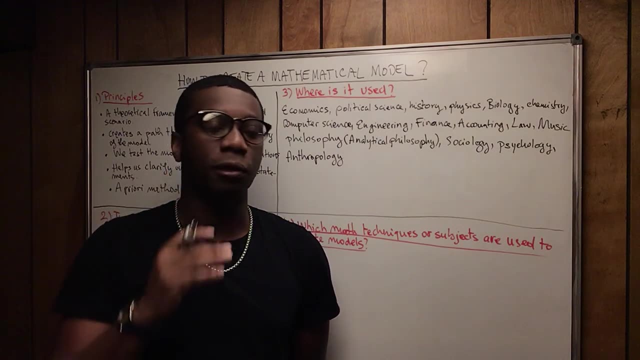 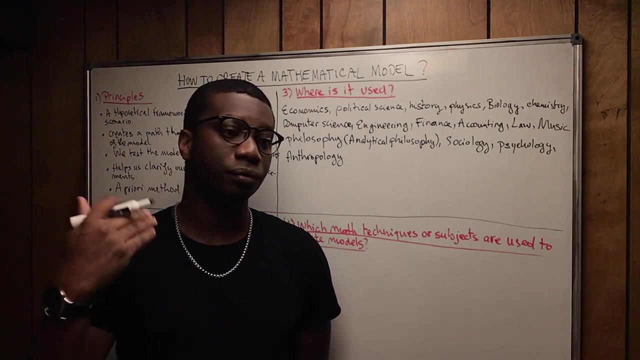 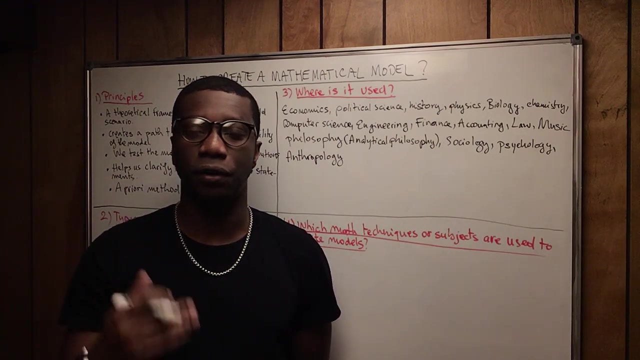 have, of course. so it is important to understand that a mathematical model does not need to be extremely complicated and the level of difficulty of the model is based on the real world scenario you're trying to describe or you're trying to predict. if the scenario touching you're analyzing is very 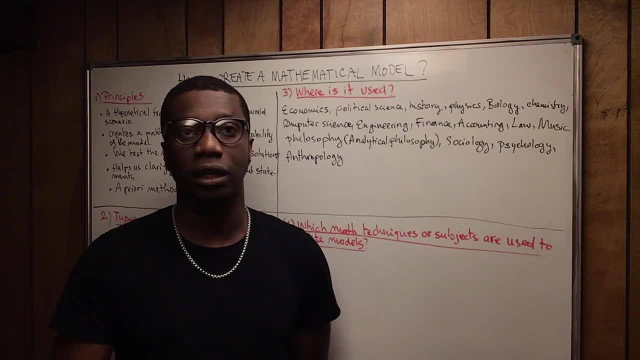 complicated scenario, then your model is going to be complicated. for recent it's the black soul's model for option pricing. it's a very complicated model that use a lot of partial differential equations. but it's because in order to set those option pricing there is a whole complex mechanism. you have to go. 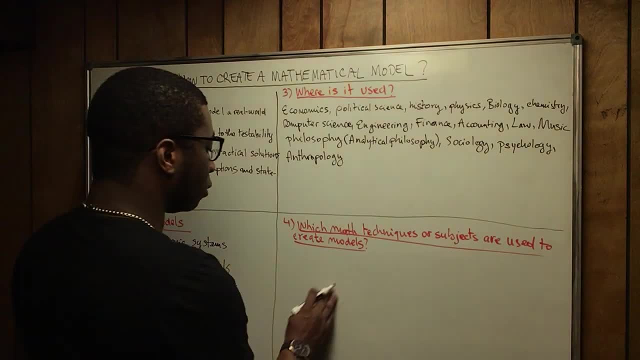 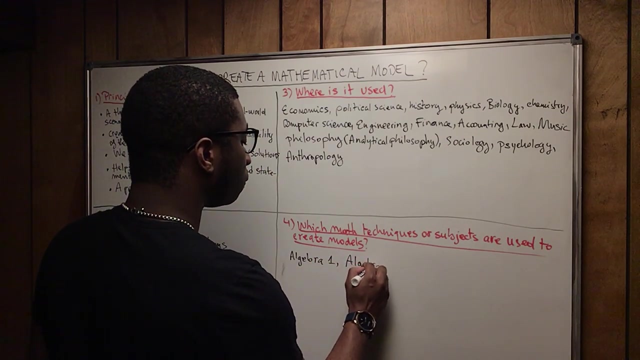 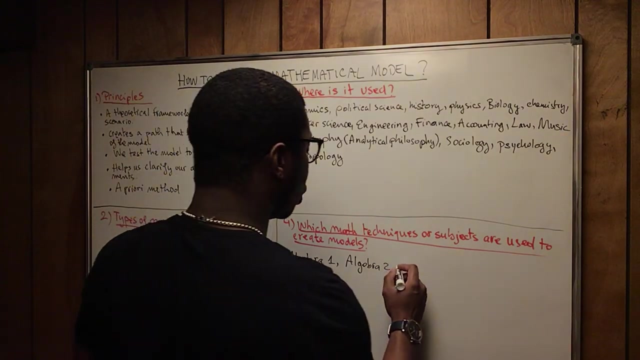 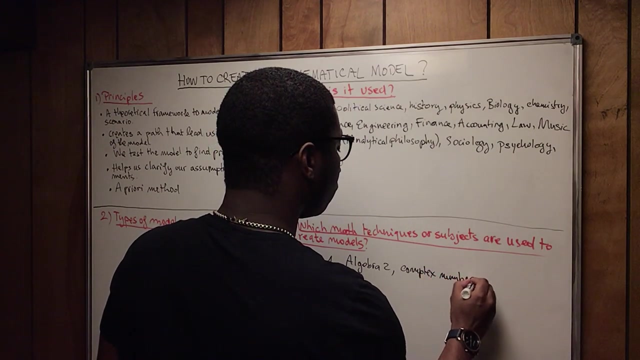 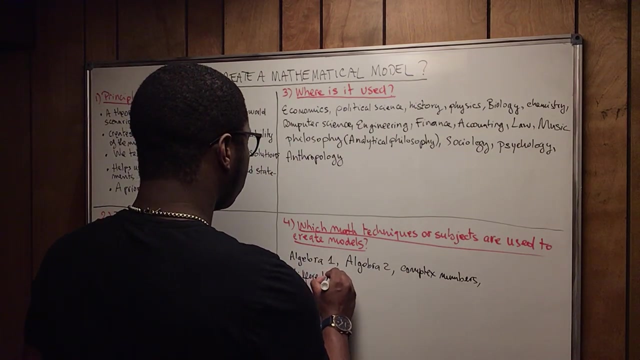 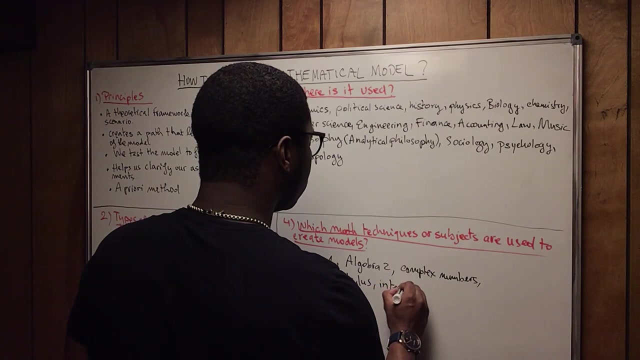 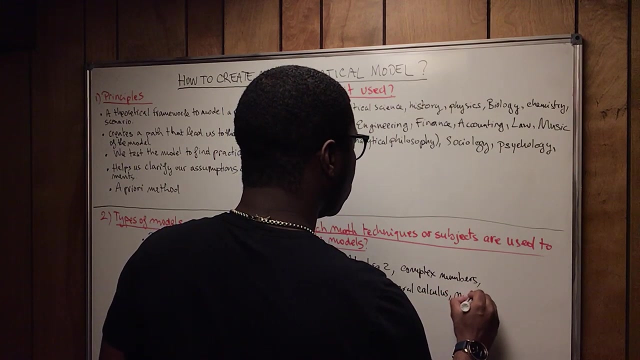 through. but a mathematical model can simply start with algebra one. okay, algebra two. you can also use some notions in pre-calculus, such as complex numbers, differential calculus, so such as derivatives, integral calculus. you can use the other different notions as seen here, so almost anyyk. 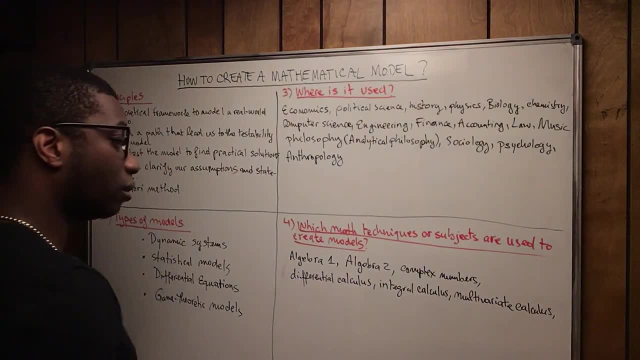 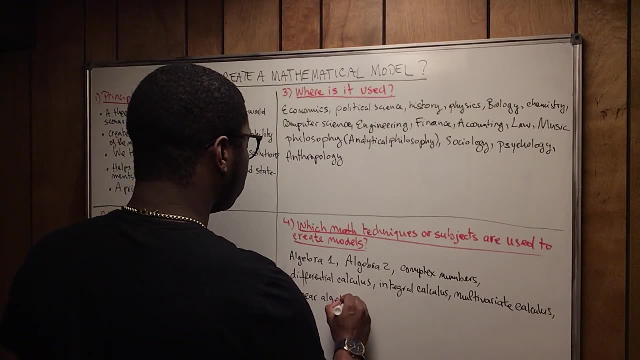 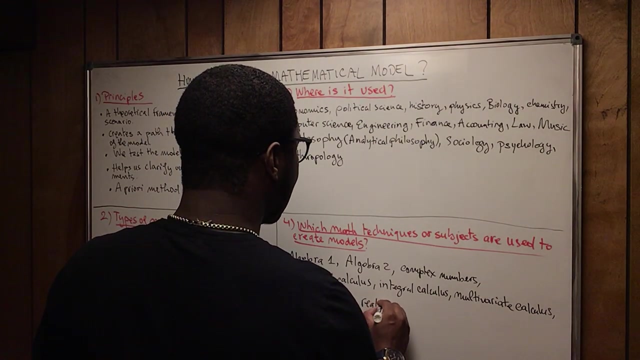 Multivariate calculus, which is normally no kalkulus. three Multivariate calculus, linear algebra. ok, this is for matrices. you can use it for real and you can use real analysis too. real analysis is: the classappy class faisait by yourivel is the same as an algebra classvenant one you can see here. okay, women Expedia. 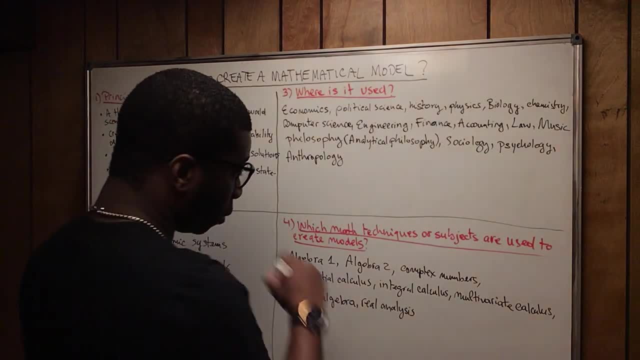 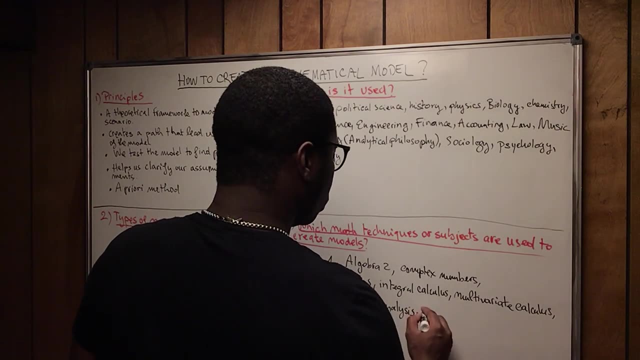 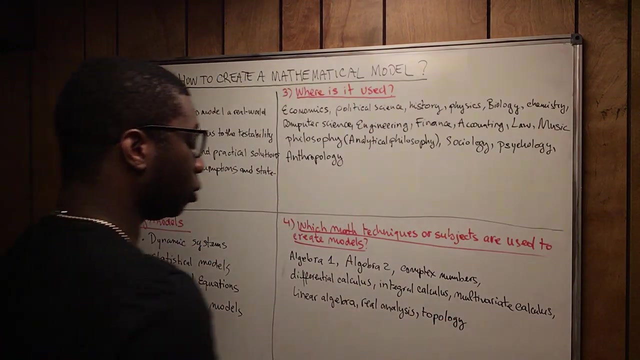 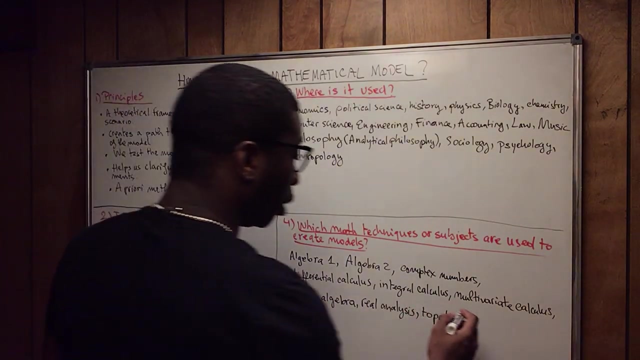 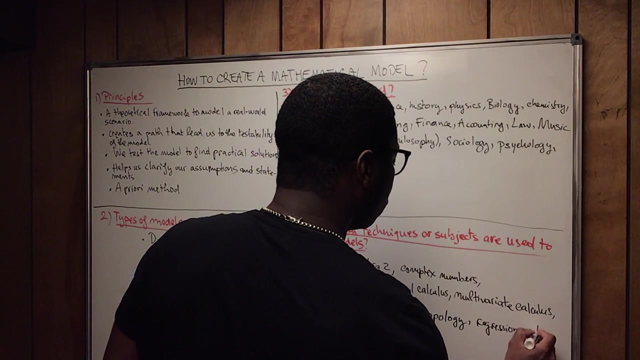 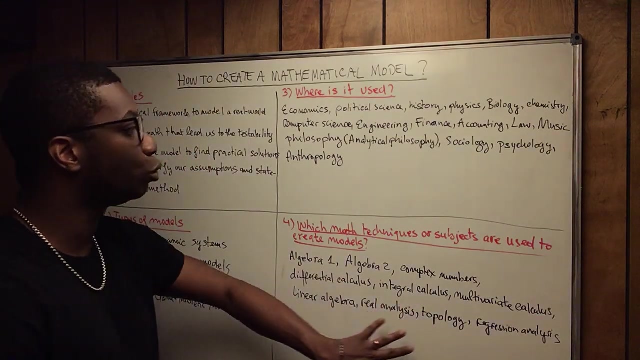 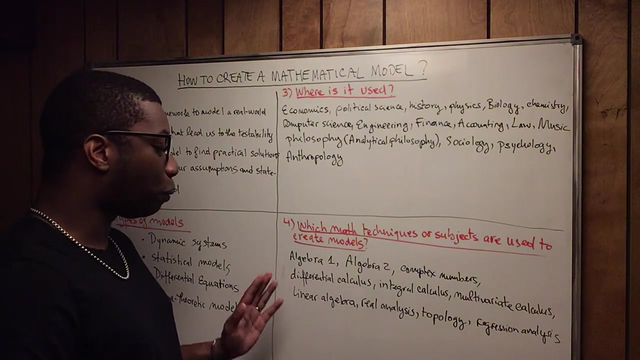 Real analysis is something I need to dive into because I have no notion of real analysis yet. You can use topology. You can use topology. You can use regression analysis in statistics, Regression analysis. So yeah, these are some of the techniques that you use to develop your mathematical model, But again, it is important to understand that everything is based on the real world scenario you are describing. 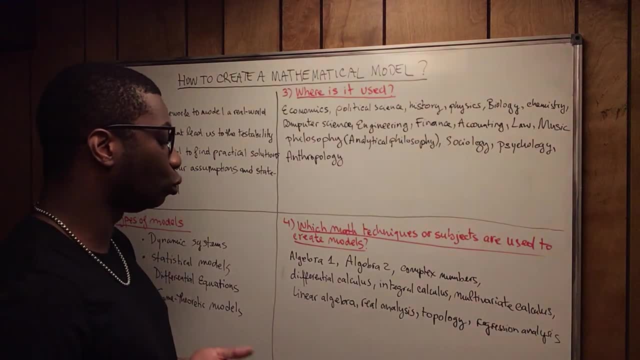 So let's say, for instance, that you are trying to use a mathematical model based on a differential equation. In order to use differential equations, you have to know differential calculus and integral calculus, specifically integral calculus. You cannot do differential equations without knowing integral calculus. It is impossible. 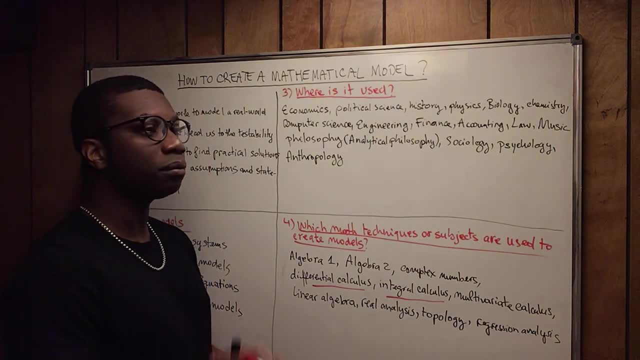 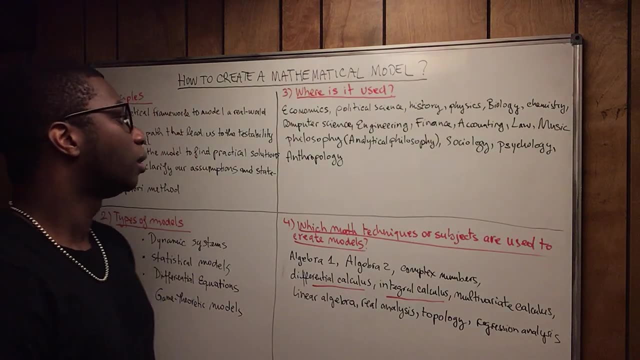 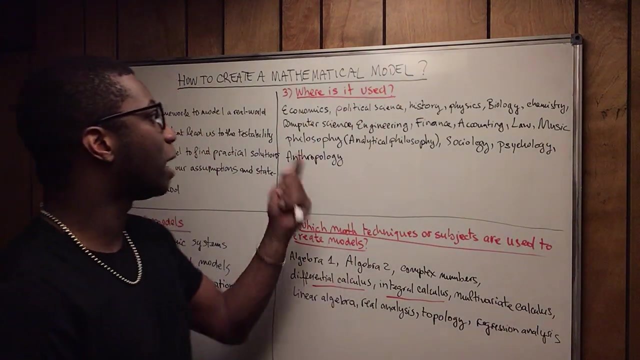 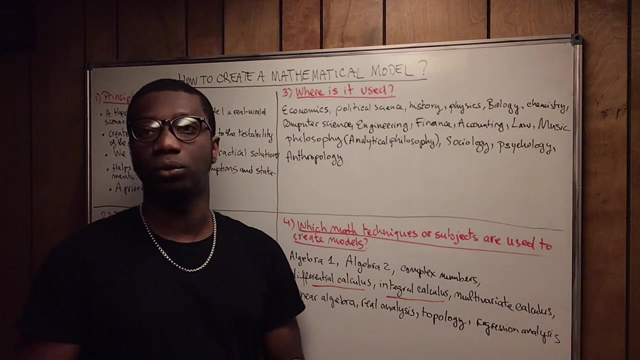 So you need basically to upgrade your math skills and then you are pretty much good to go. So Where- and let me say in which industry mathematical models are used? They are used everywhere. In fact, industries use it every day to determine how they are going to allocate their resources. 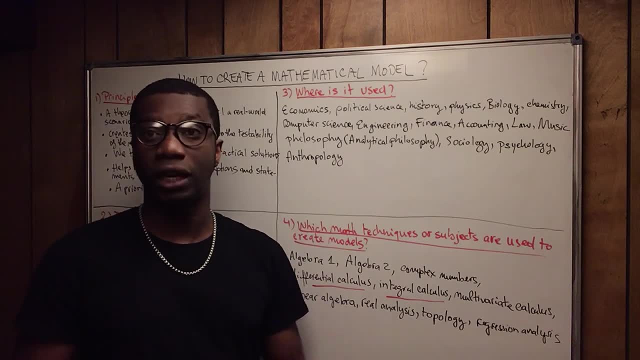 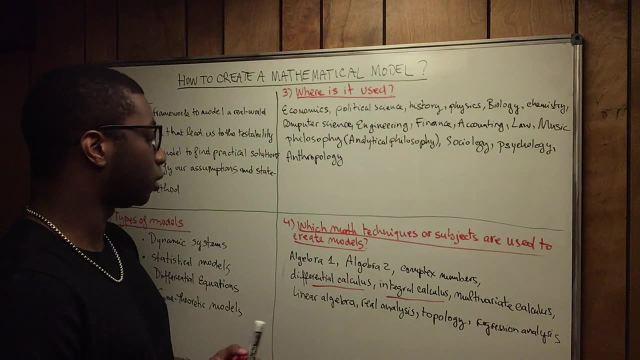 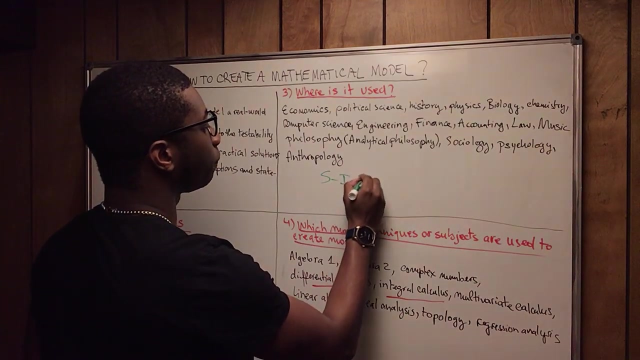 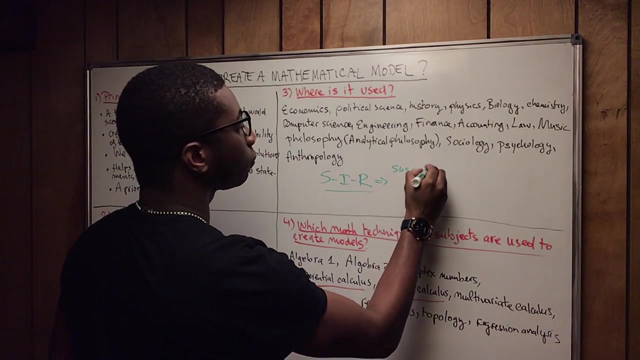 In healthcare. it is used to determine the spread of disease and how to contain that spread. In fact, there is a very famous mathematical model used in biology called the Sperm, The Sperm model. okay, the Sperm model stands for people who are susceptible to be infected. that's what the S stands for. okay. 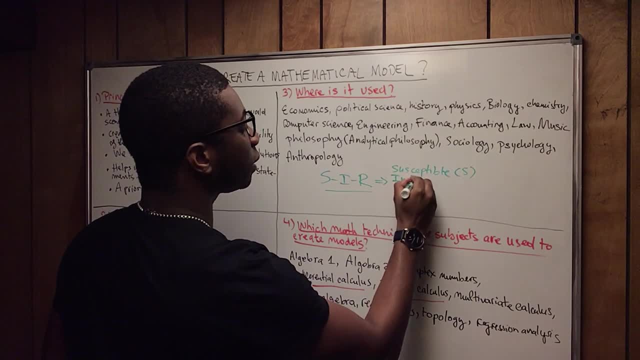 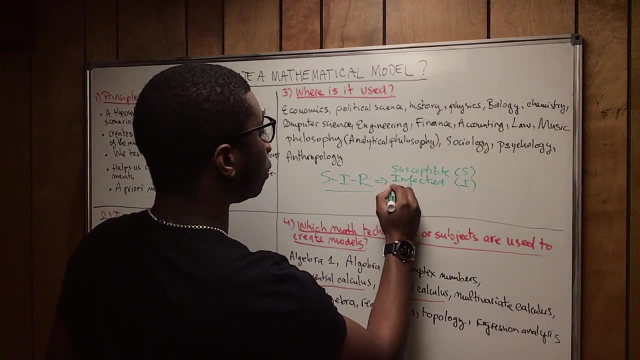 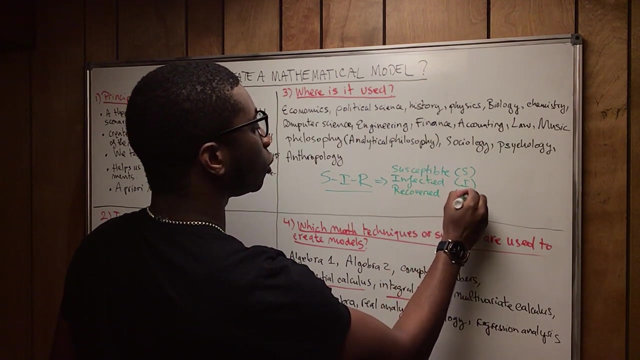 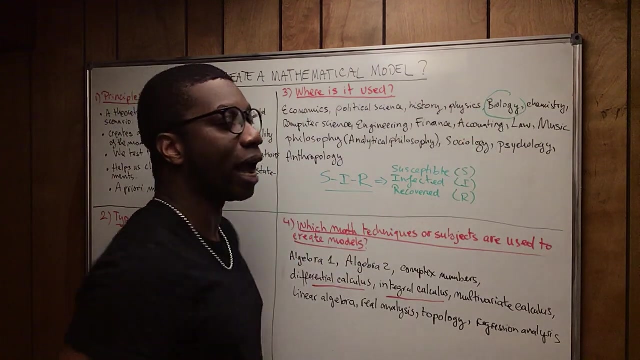 The I stands for infected people, who are already infected by the disease, And then you have the R for people who have recovered, So who can no longer be affected by the disease. So the Sperm model is used in mathematical biology and even in medicine. 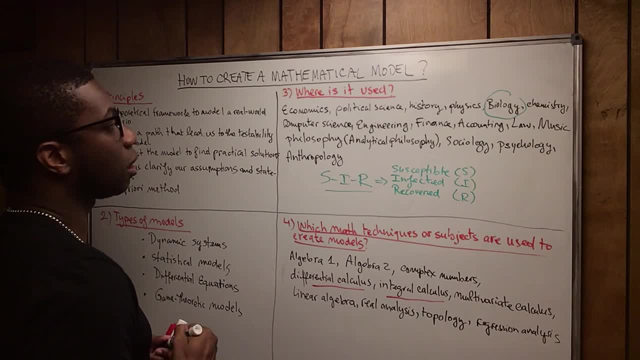 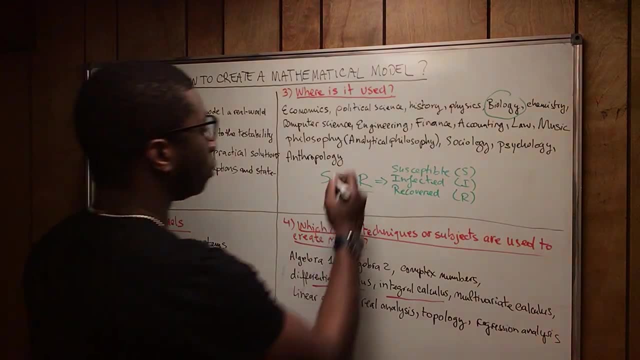 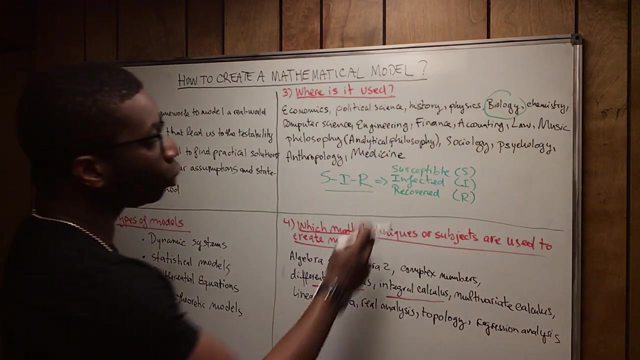 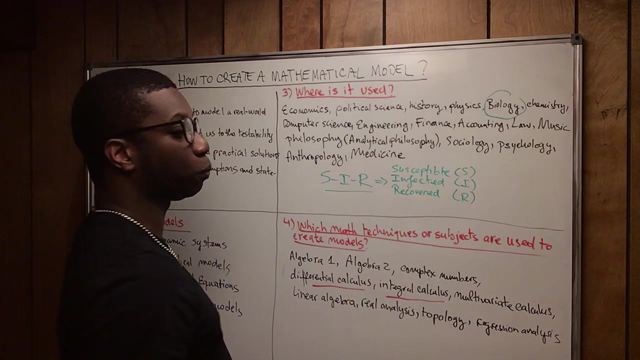 Oops, I even forgot, Now that we are coming back to the fields where it is used. You have medicine. Forgot about this. Okay, So you have medicine. So this is used in healthcare to determine how disease are spread and contained? okay, 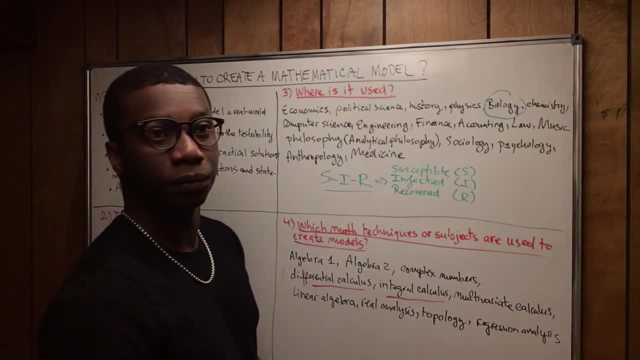 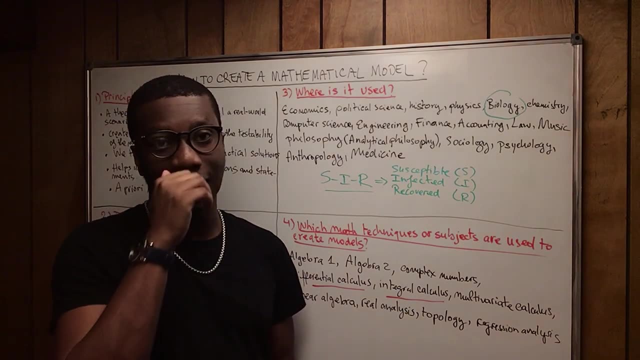 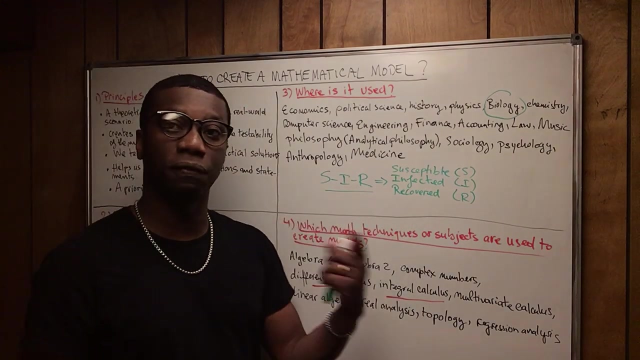 And that's the model they use, for instance, for COVID: to determine where COVID is going to go, how we can contain it and the vaccines, that, and they develop a vaccine accordingly to the SIR model. So, and that's even how I learned how to develop mathematical models using differential equations. 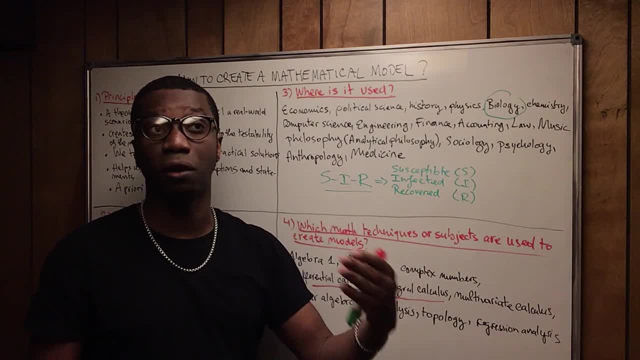 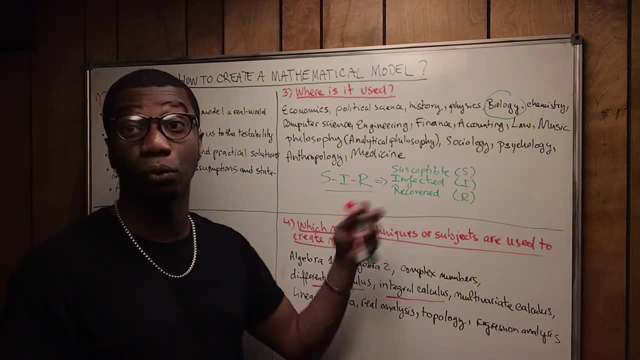 The SIR model. if you don't know how to use this, there are many videos on YouTube where you simply type mathematical model and the SIR model is one of the first videos that will appear when you're looking for mathematical model videos. okay, 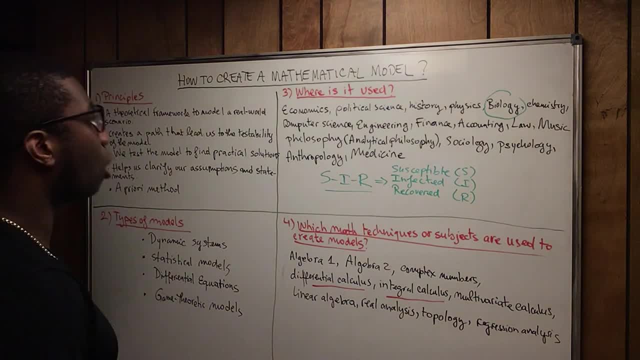 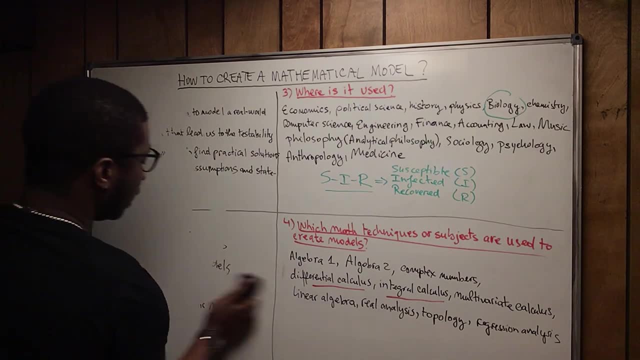 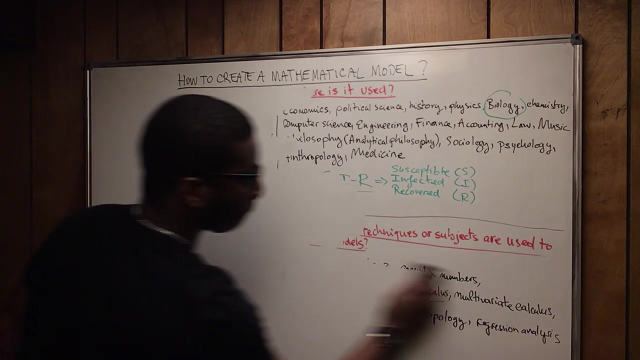 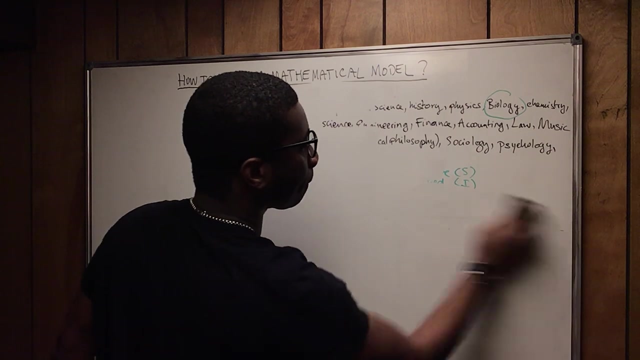 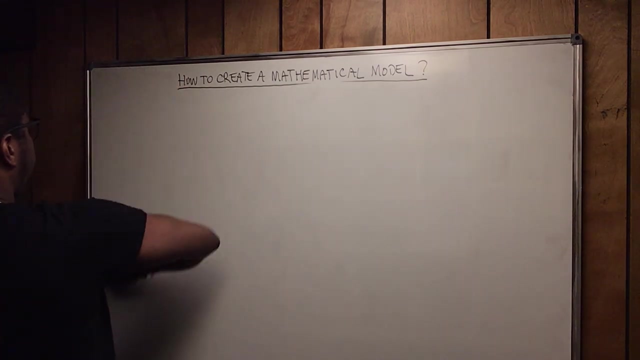 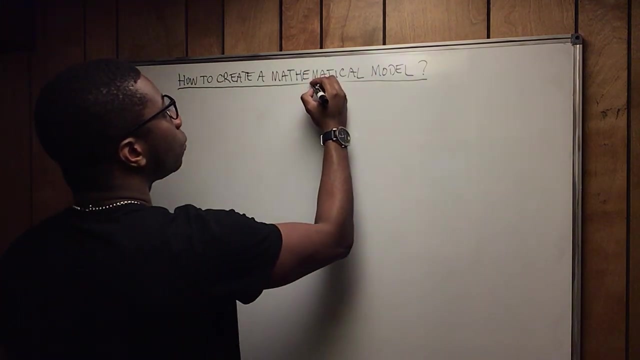 So now I'm going to show you the process of mathematical modeling, and then I'm going to give you a very simple example, and then that's it when we will talk about mathematics. All right, Okay, so here we are going to deal with. 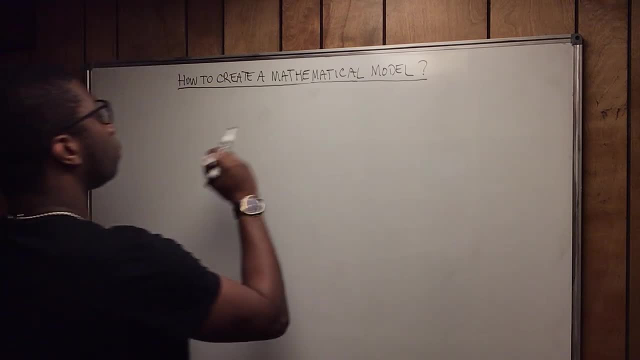 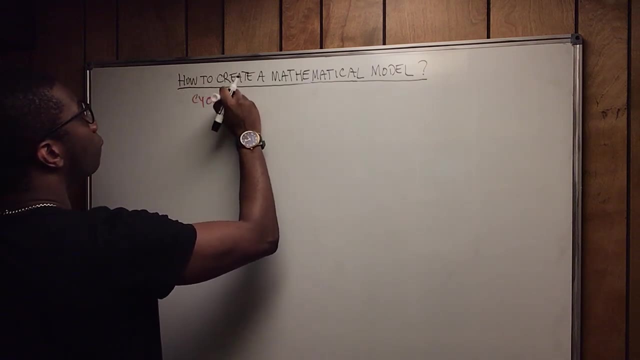 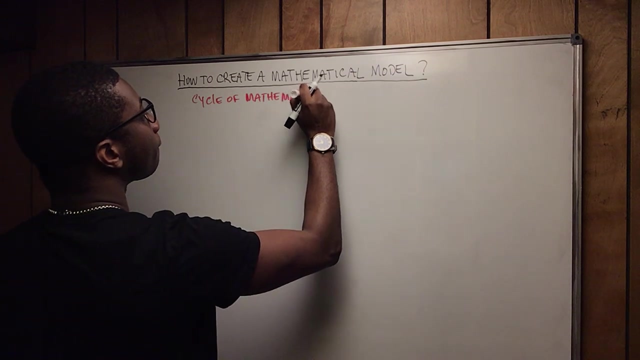 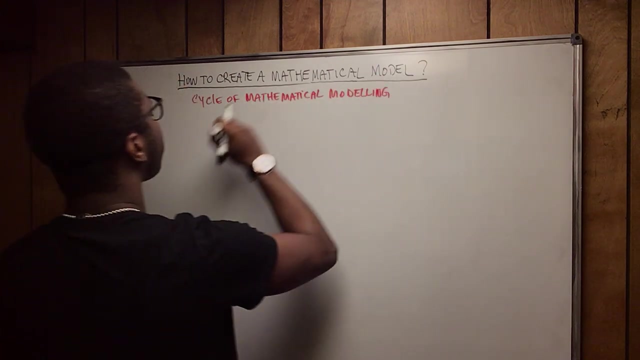 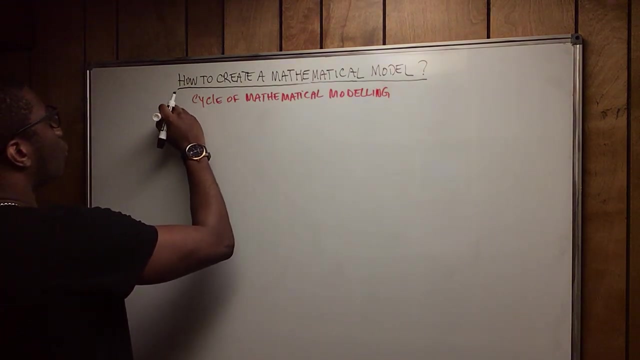 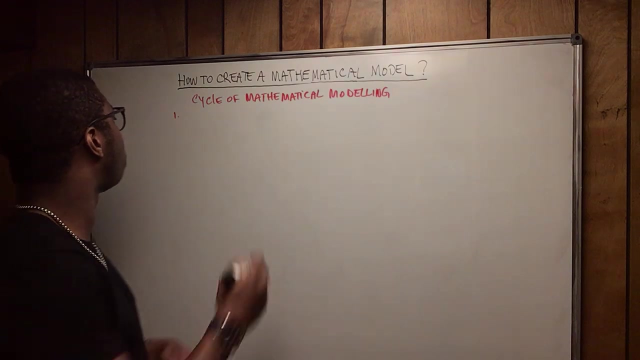 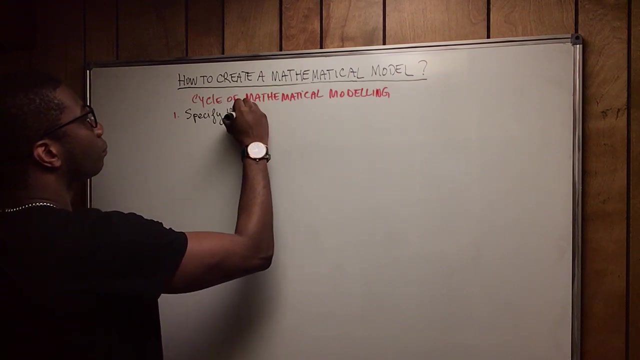 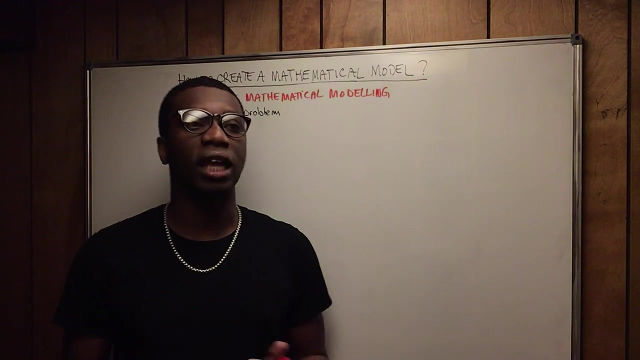 sweat hands for some reason. we are going to deal with the cycle of mathematical modeling. so the cycle of mathematical modeling is based on seven steps, so one one is basically to specify the problem. so you got to specify your problem. you got to say: what am i talking about? what is the real? 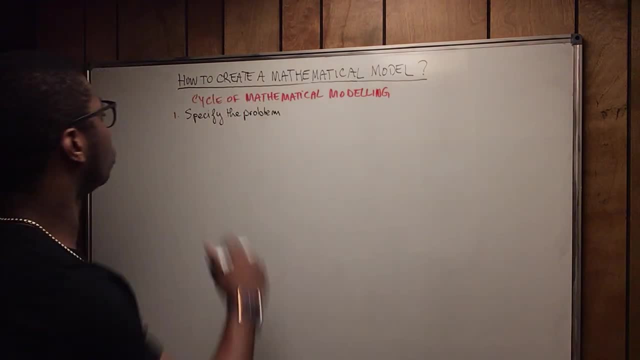 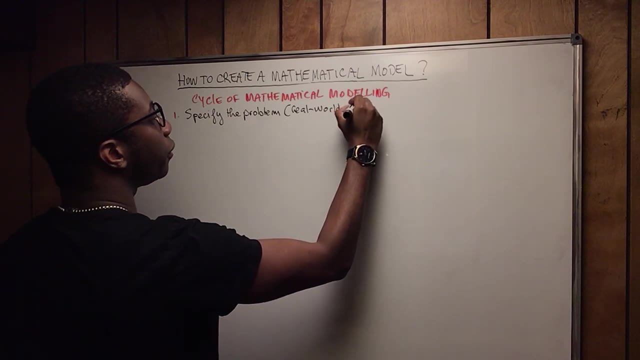 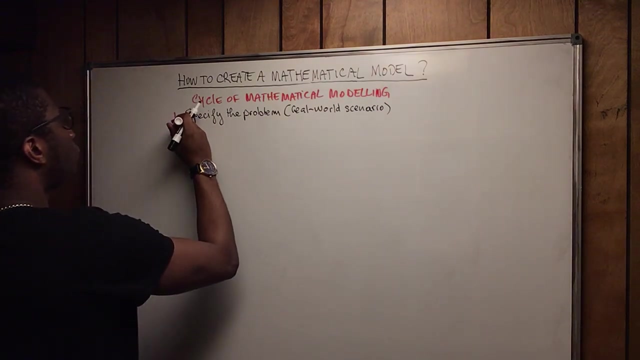 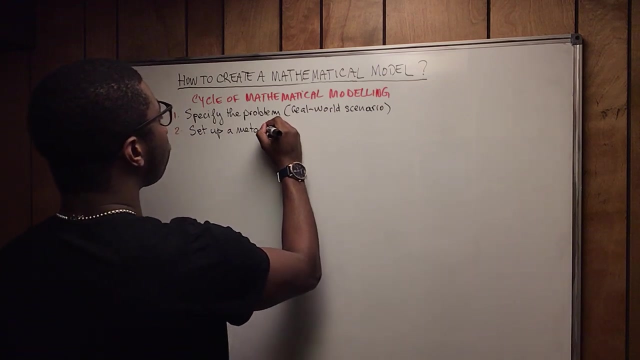 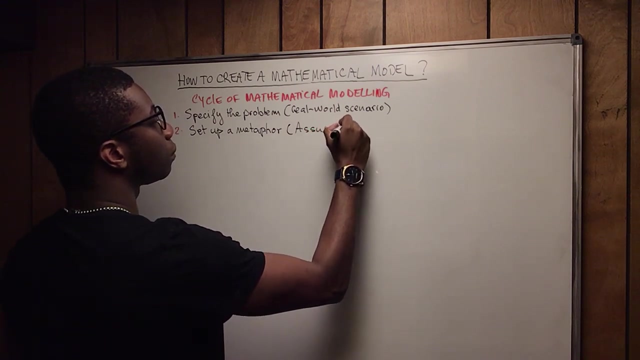 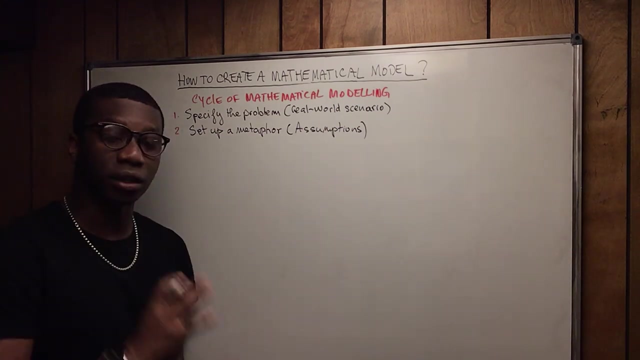 world scenario am i describing right? so specify the problem. that's the real world scenario. okay, two, you gotta create, you gotta set up a metaphor, set up a metaphor. so set up a metaphor is the most crucial part. your assumptions, okay, your assumptions, that's where you actually building the model verbally, that's where you 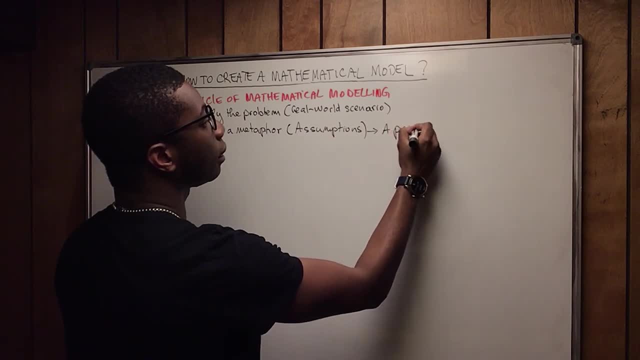 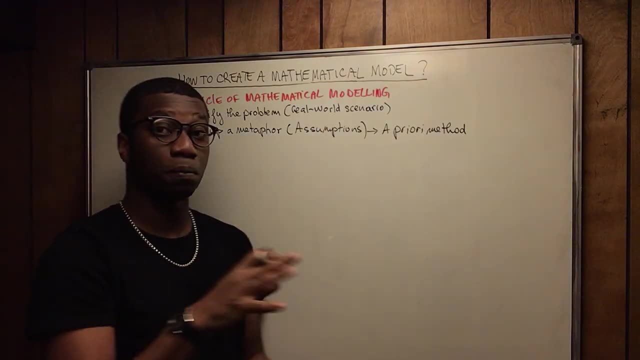 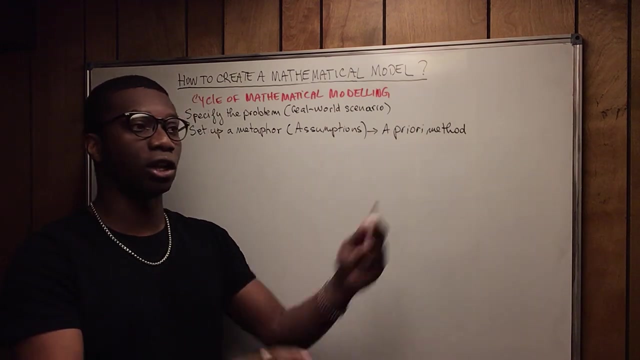 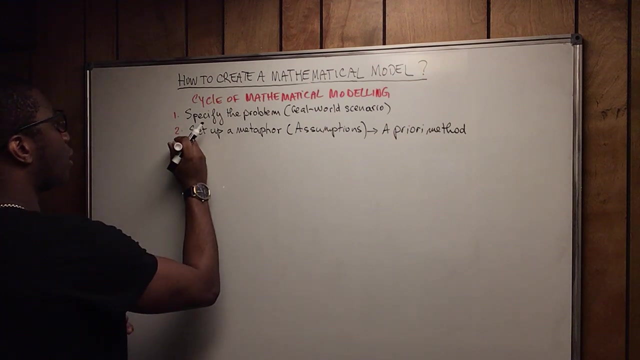 use a priori methods. okay, that's what you're building, your model verbally, you said. you basically saying this occurs. this occurs because of this. therefore, if this happened, then this could happen. that's the part where you set up the metaphor, and then here three. that's when you formulate: 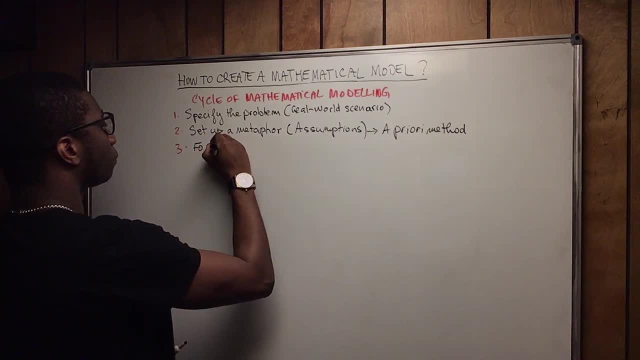 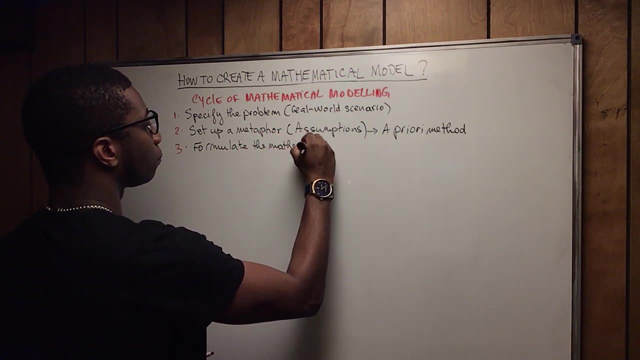 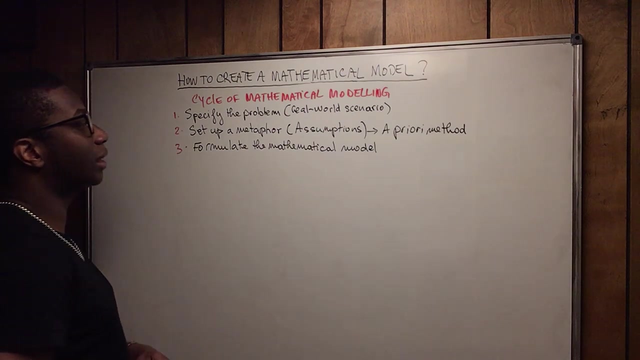 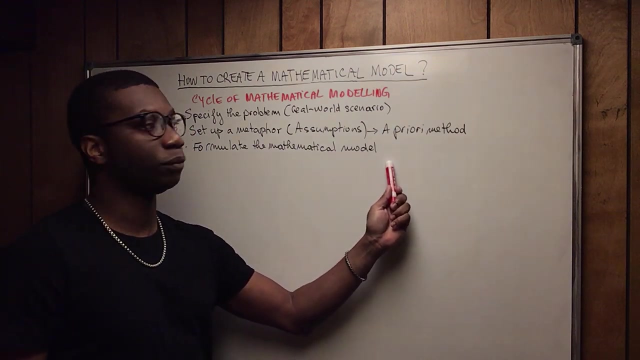 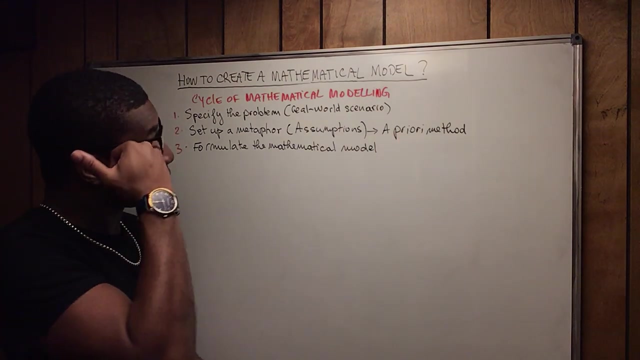 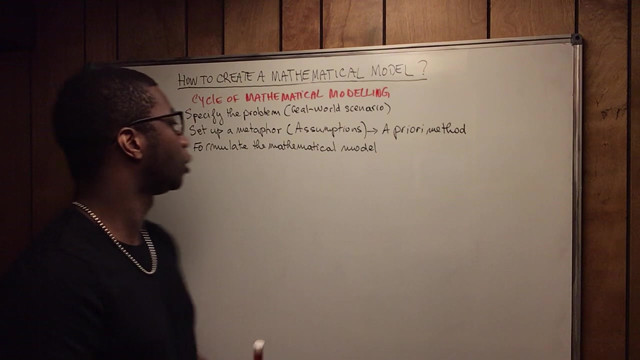 the mathematical model. That's where you are basically transitioning the verbal reasoning into mathematical reasoning. So you're transitioning from the verbal language to the mathematical language. When you say it in your assumptions verbally, you write them into mathematical language in a form of equation. 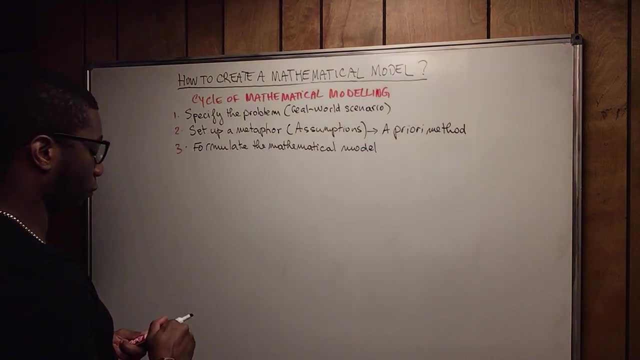 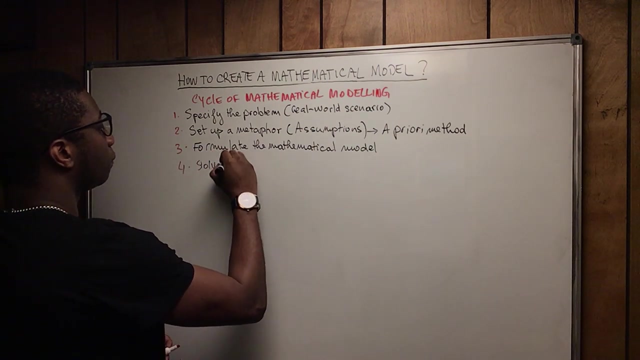 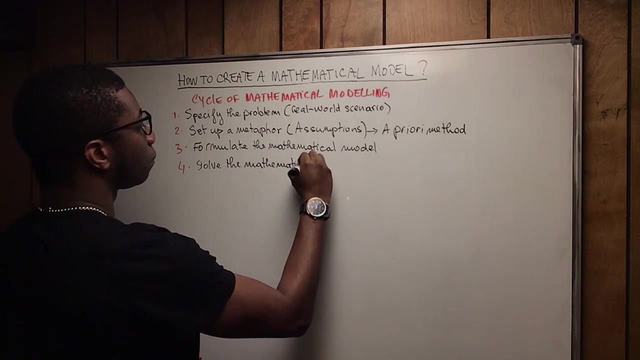 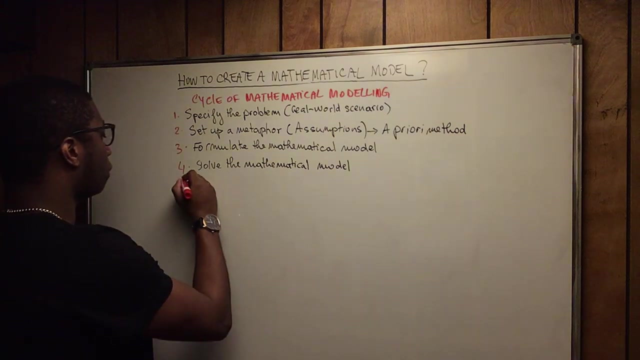 Then, for you are going to solve the equation, you're going to solve, solve the mathematical model. you're going to solve the mathematical model. you're going to interpret the result. you're going to interpret the result or the results, It depends. 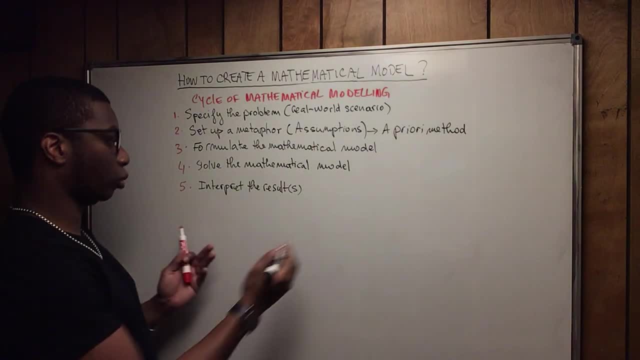 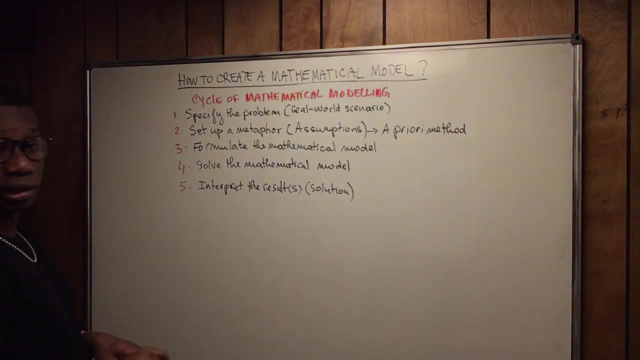 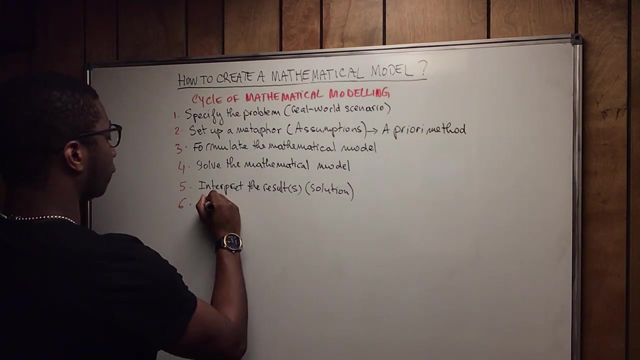 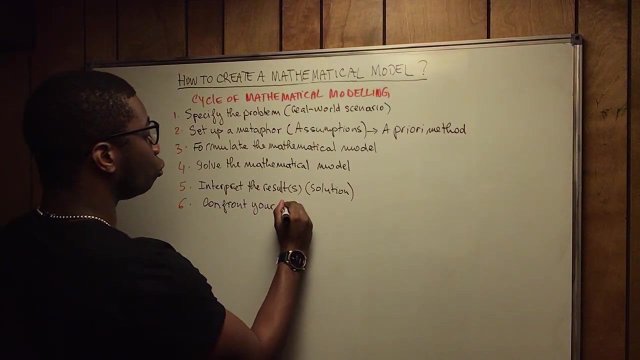 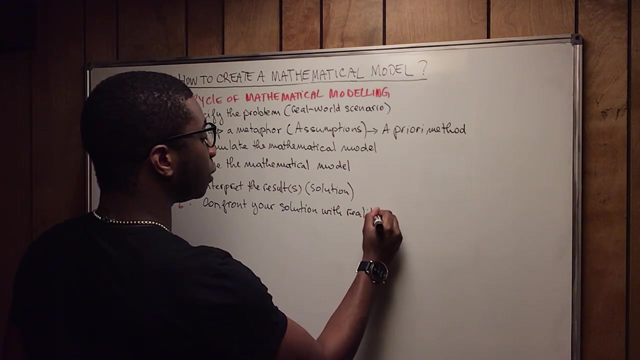 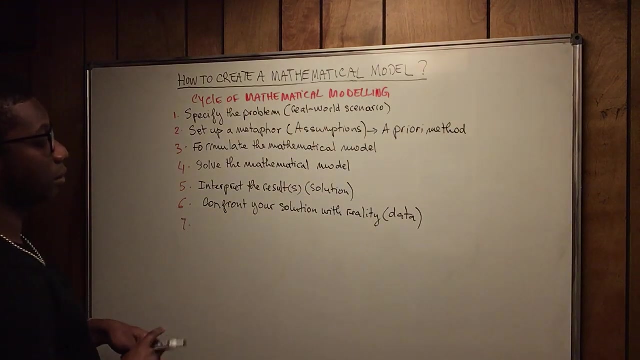 Okay, Okay, It depends on the solution. And then six: you're going to compare your results with reality. So let me put it here: confront your solution with reality. Okay, Okay, Okay, Okay. And then seven: you have to use it to explain, predict and to calculate. 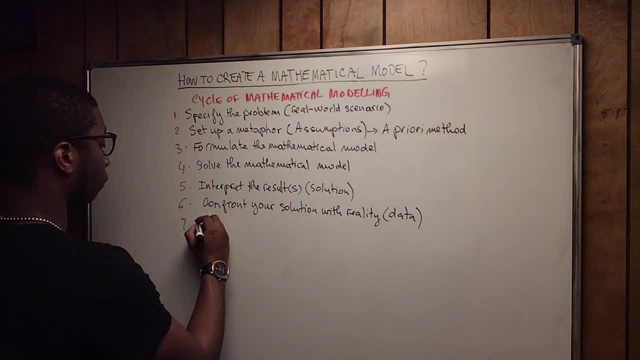 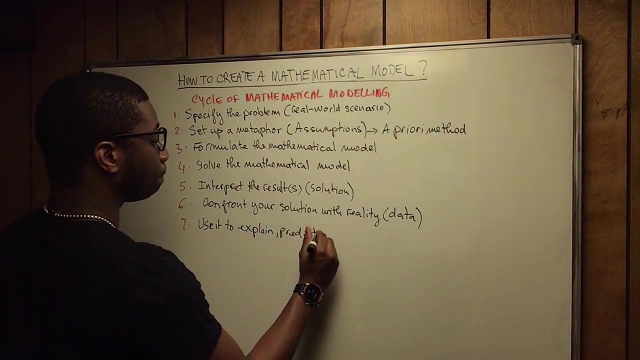 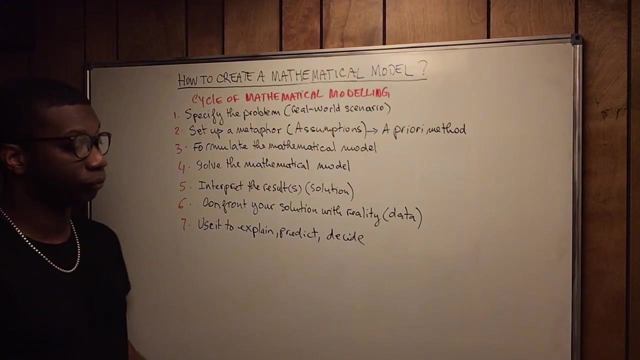 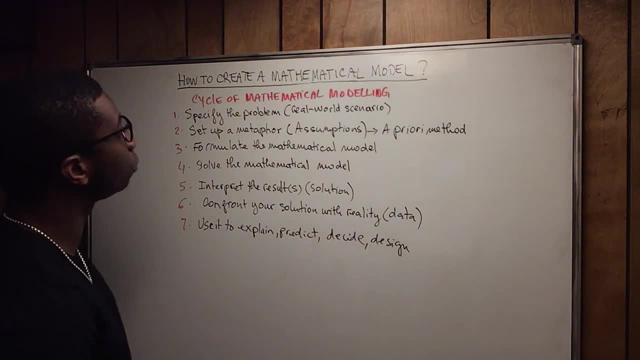 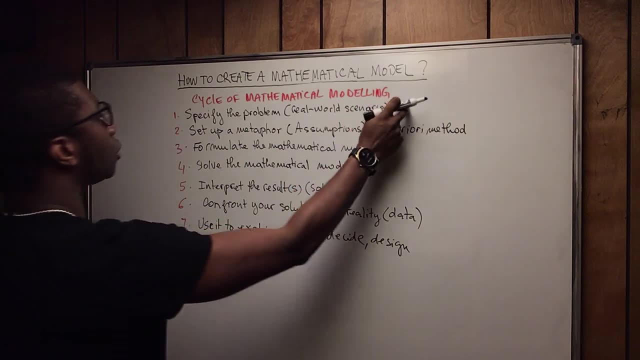 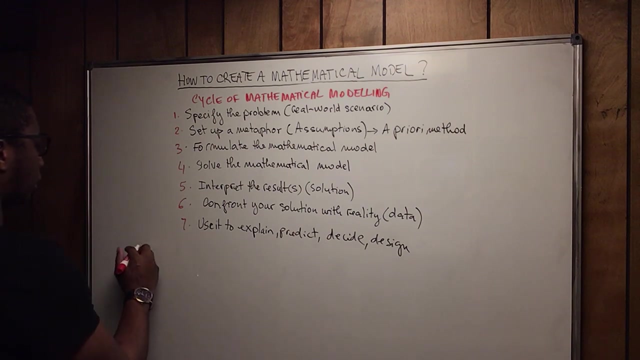 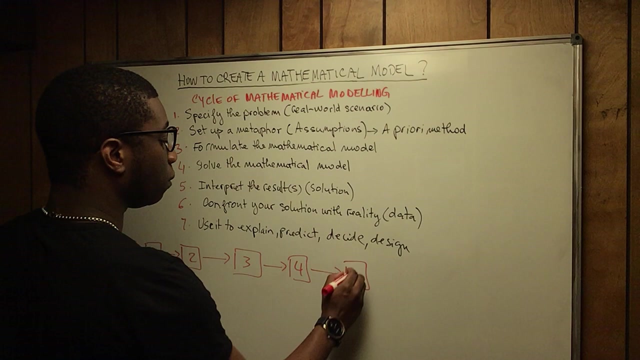 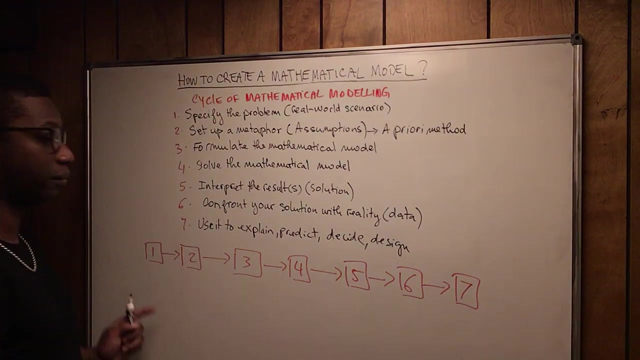 there we go. that's how you develop a mathematical model, okay, so let me try and put it so you first start with by specifying a problem, so it's it goes like this: okay, one, two, three, four, five, six and seven. that's your mathematical model. oops, let me put it so you don't think it's a 16, okay. 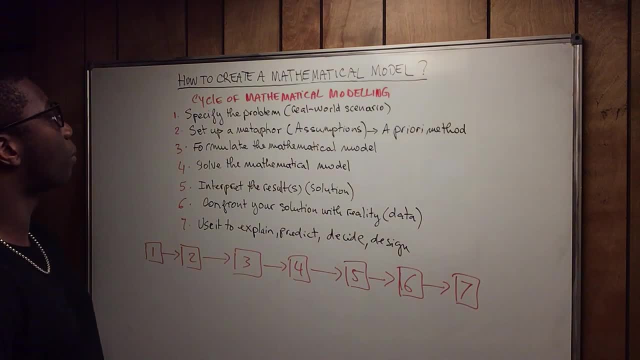 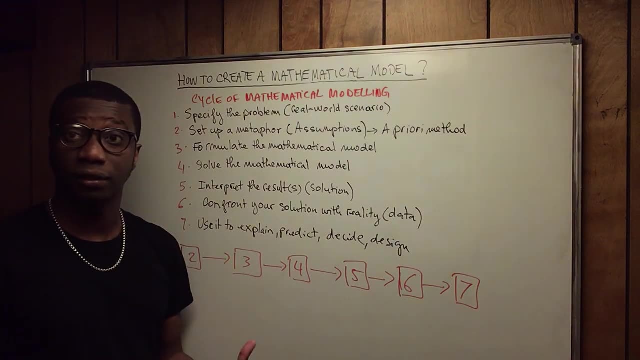 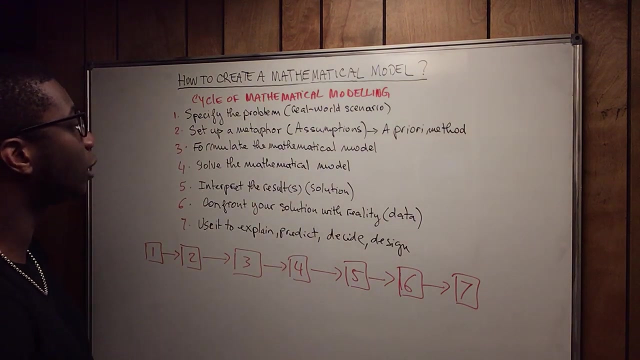 so this is the cycle of a mathematical model. so you first specify the problem, so you describe the real-world scenario that you're trying to understand and solve. you set up a metaphor. the number two to me is the most crucial part, so I'm putting this star here. it is crucial. 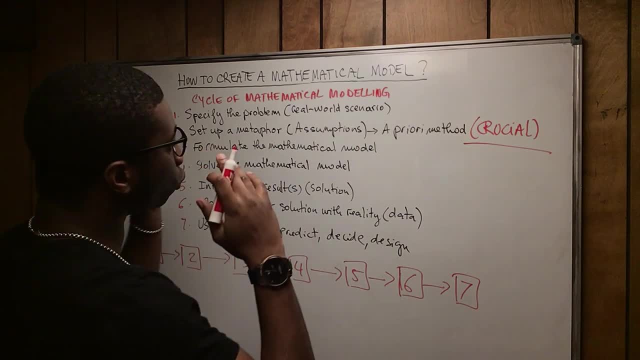 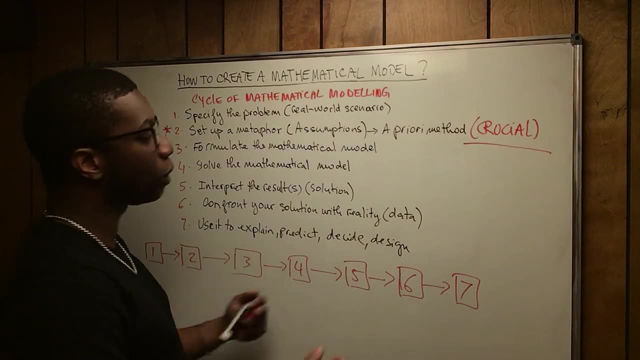 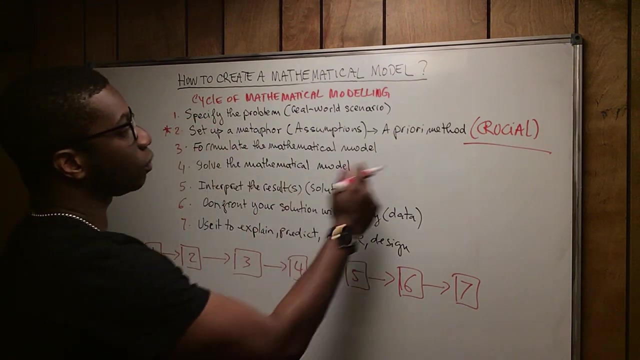 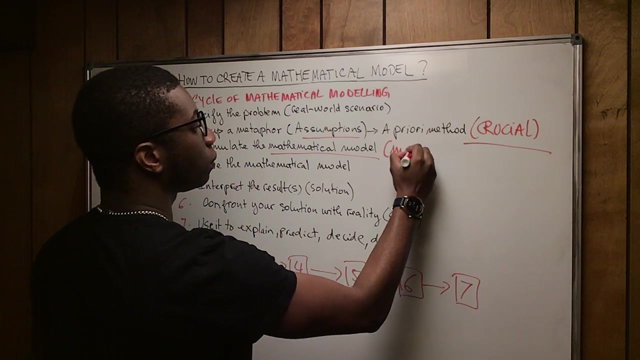 you set up a metaphor. so basically, you create a, an apriori framework that you create, if the reticle framework based on the apriori method, and then you move to the third part, which is to formulate whatever you describe here in this in a mathematical language. 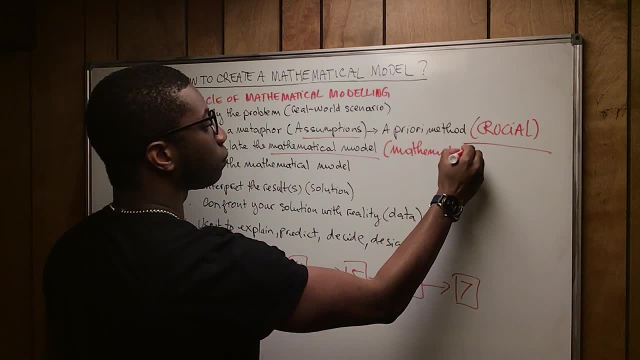 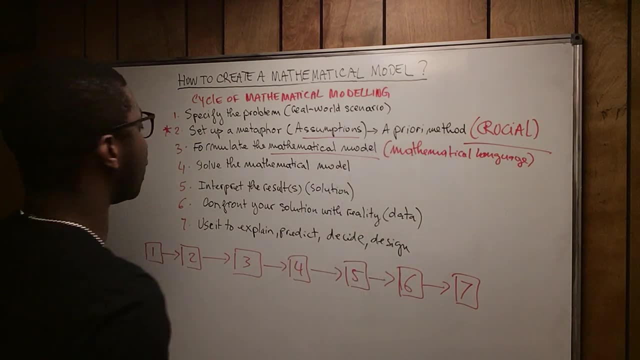 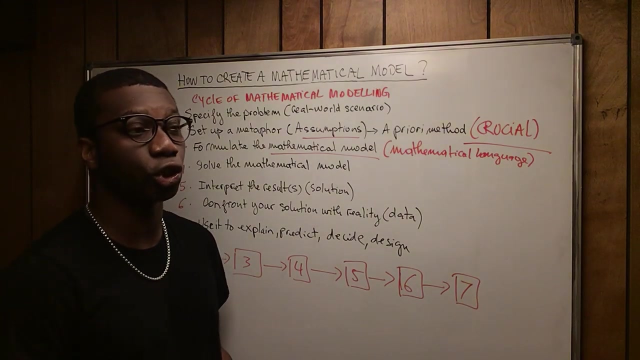 you. okay, you describe that into a mathematical language and then you solve the model. that's where you're going to use your differential equation or your statistical model or your theoretic game or your dynamic system. it depends or it depends on the scenario you are describing. 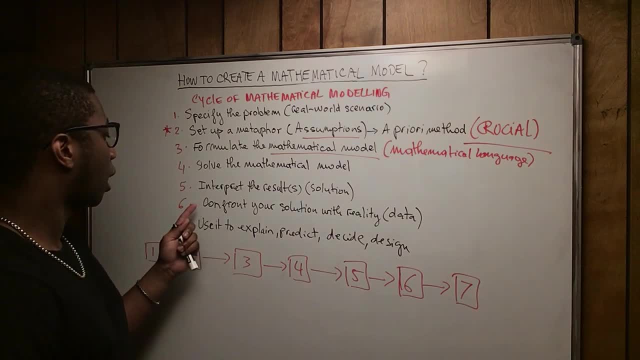 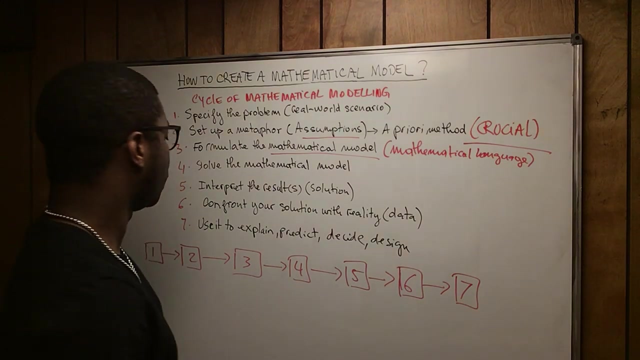 then you're going to interpret the solution, the results, and then you're going to confront that with the reality, with the data. you see if whatever model you describe con is conform with the data. if it is, your theory holds. if it's not, you gotta refine it. there's no shame in developing the wrong mathematical models. like scientists, 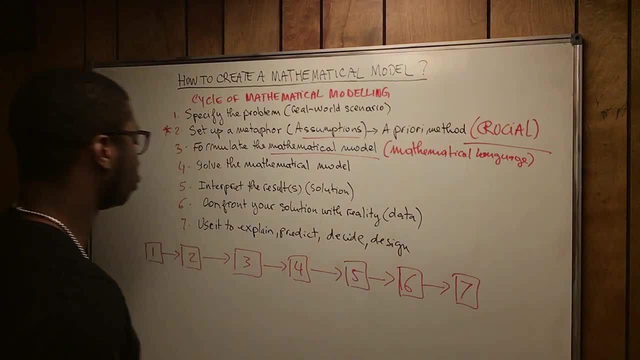 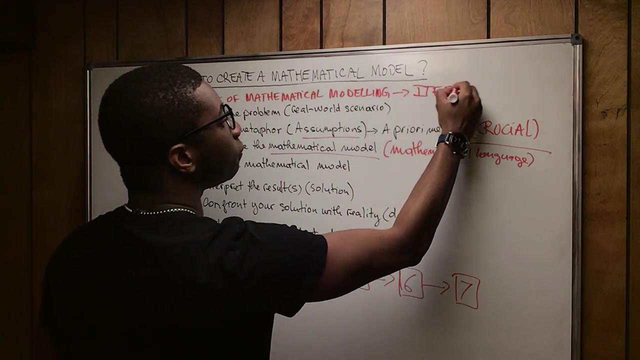 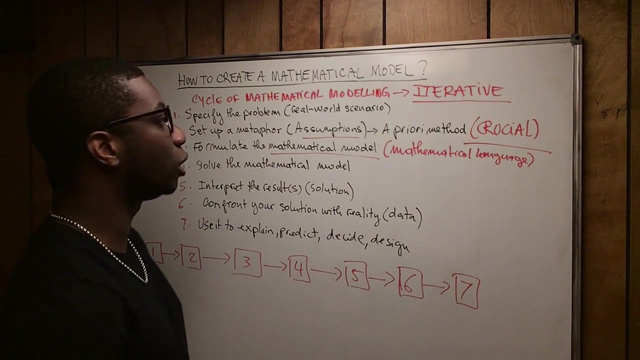 always develop wrong mathematical models at first and then you use it. you use that model to explain, to predict, to decide or to design. you need to understand that in mathematical models. so the cycle in fact is iterative. it is an iterative process. so that's why, even when you create a model, it's not done. 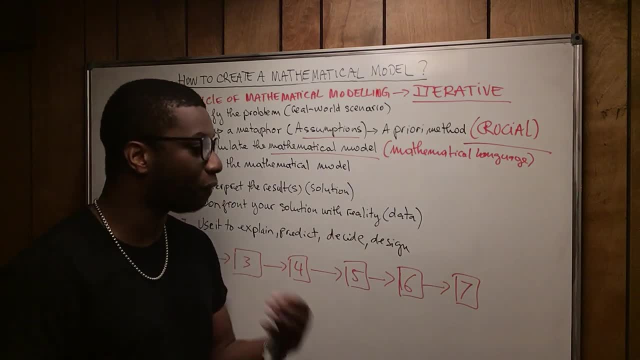 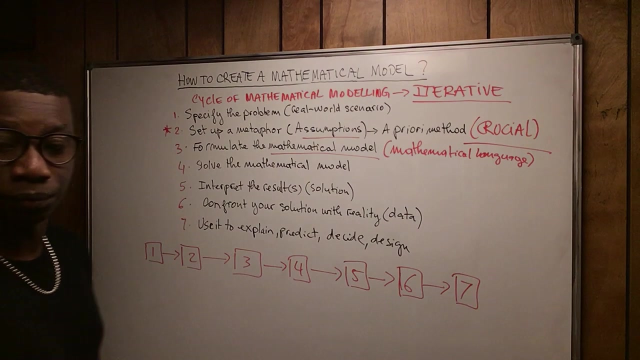 you have to refine it. even if your model is right, you still have to refine it in order to adjust it to the world, because the world is moving, so you have to constantly refine the model in order to make it compatible with the current situation. so now we are going, I'm going to show you a very 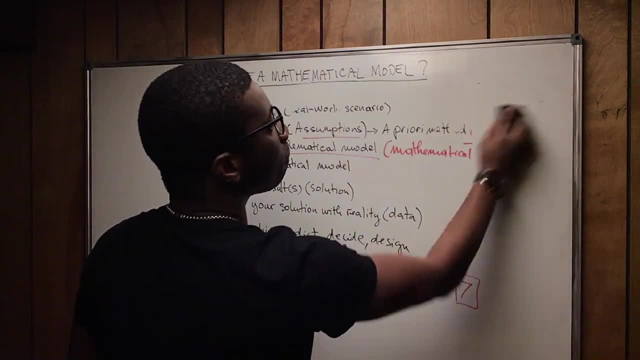 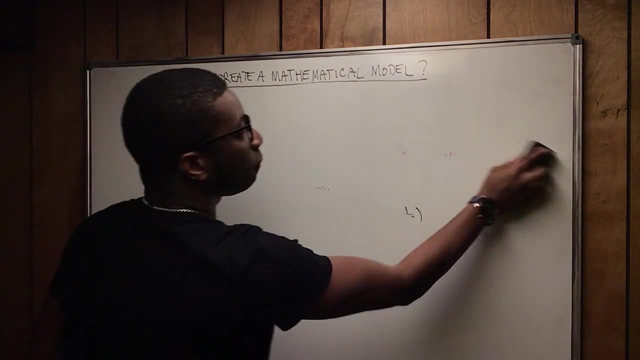 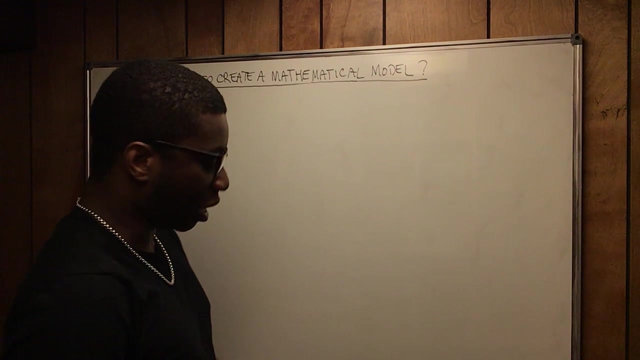 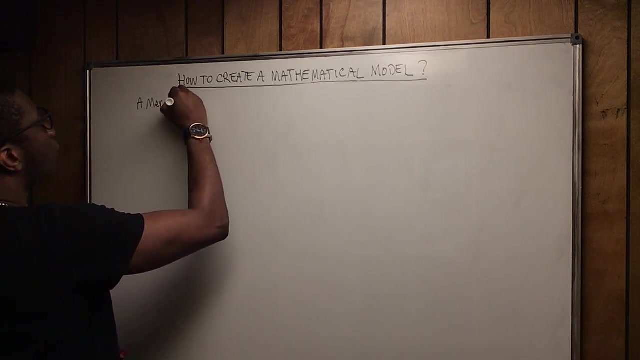 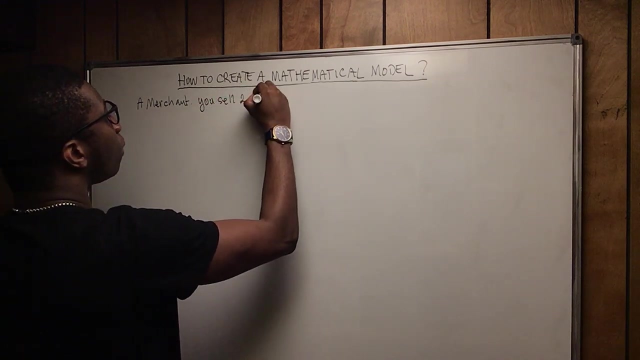 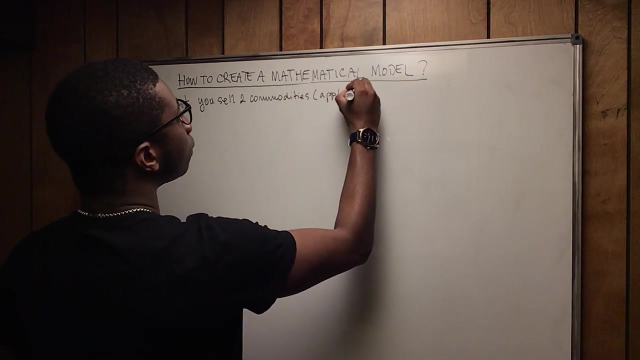 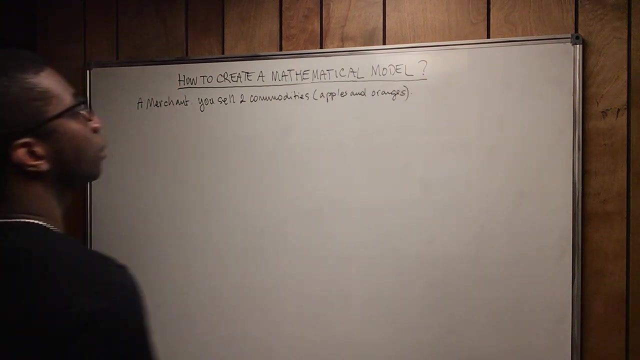 simple example of how to develop a mathematical model. so you have an idea, because everything so far I taught you here is theoretical. alright, so let us say that you're a merchant- okay, so a merchant, and you sell two commodities, so Apple and oranges. apples and oranges. okay, and you sell these into two markets. so 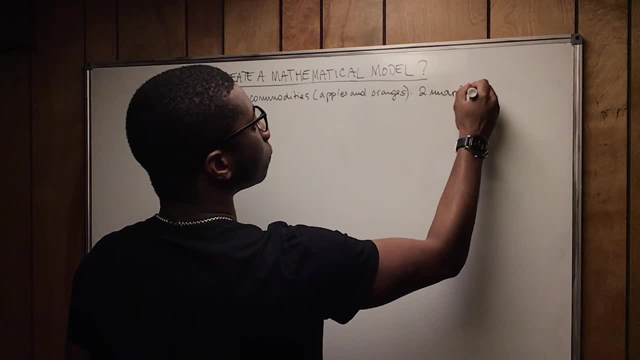 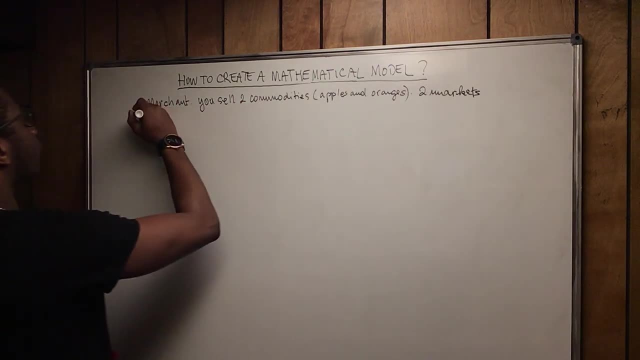 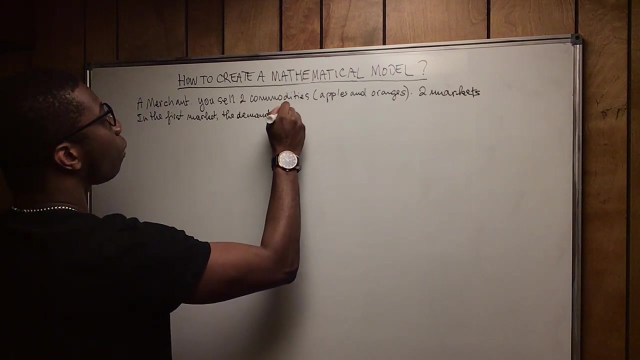 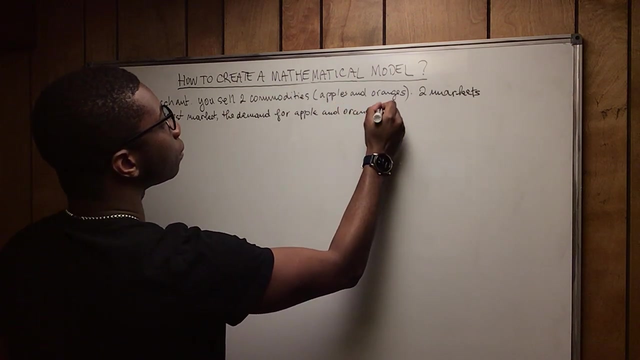 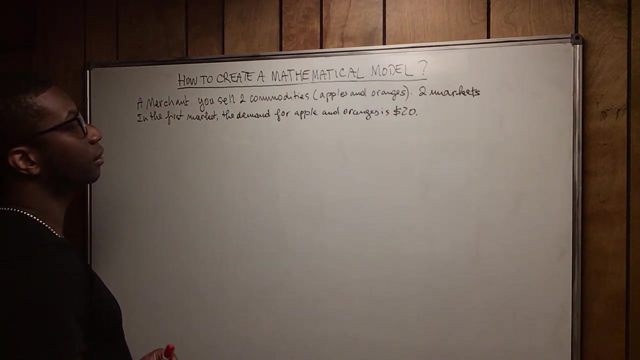 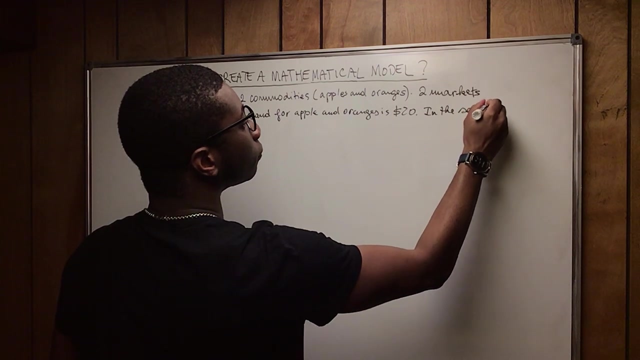 two markets. you sell your Apple and oranges into two markets. okay, in the first market the demand for Apple and oranges is about, let's say, twenty dollars, right. and in the second market is about, let's say twenty dollars, right. and in the second market, that' mint. 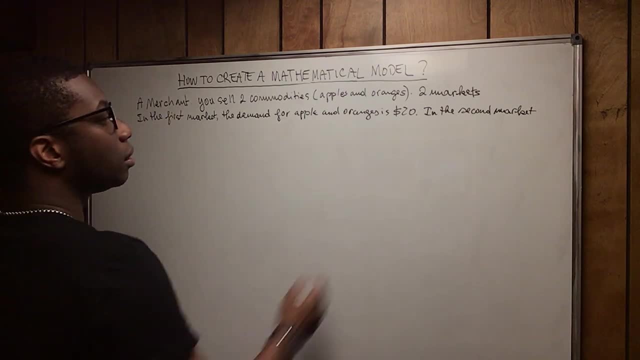 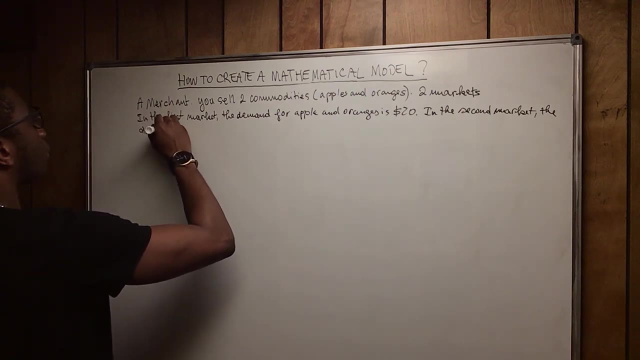 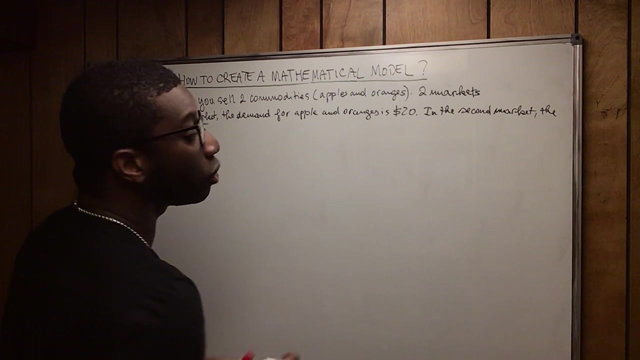 on the first market. together you can income, which means that your길 is حال is, let us say, $15 right, and in the first market, you need to produce. in fact, you don't know the exact amount of apple and oranges you need, but you need to produce. 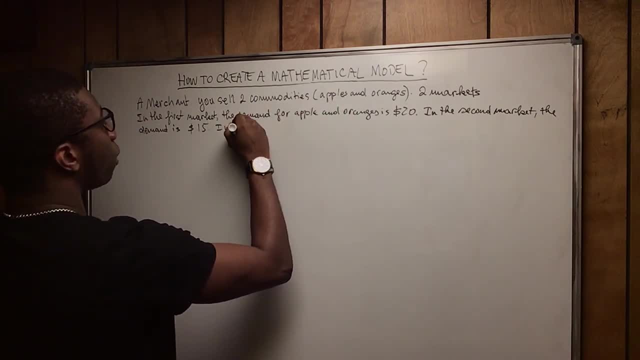 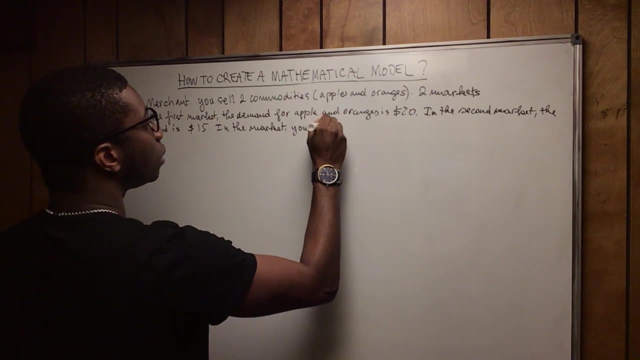 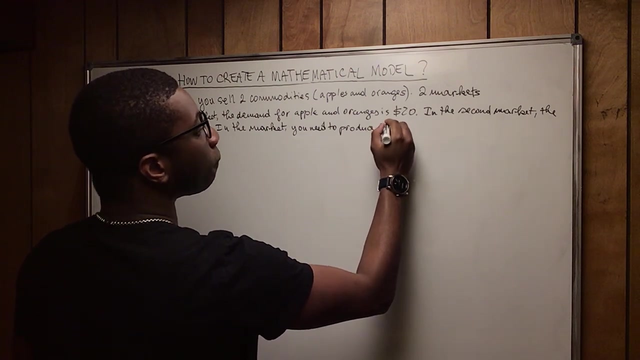 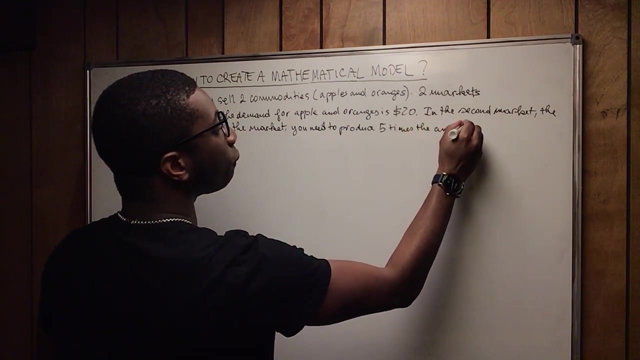 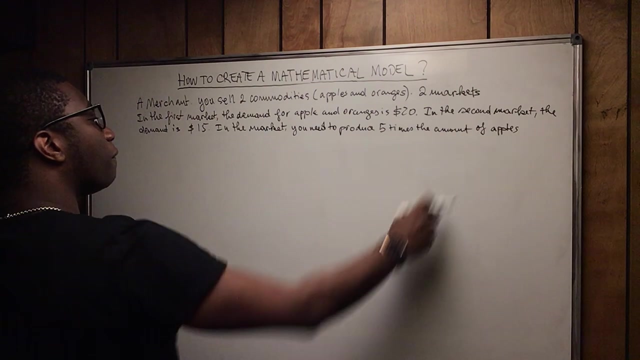 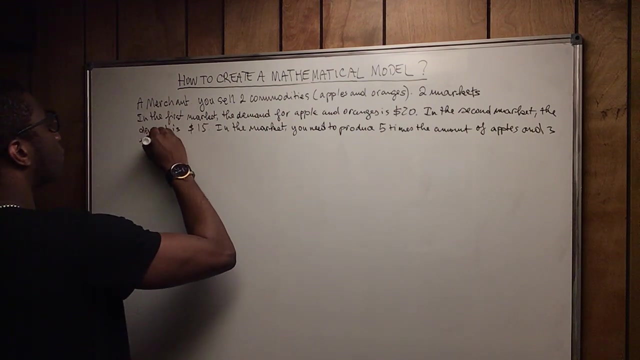 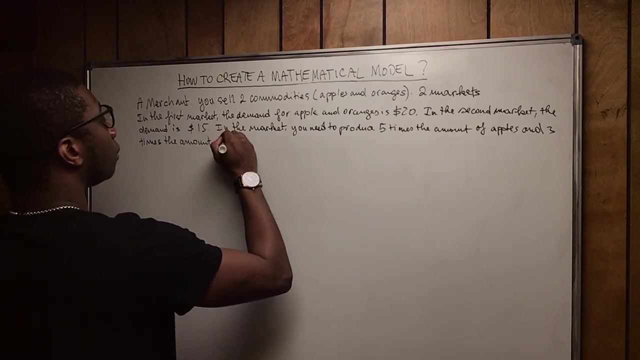 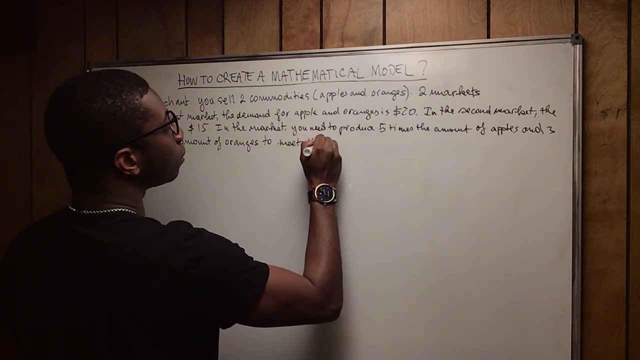 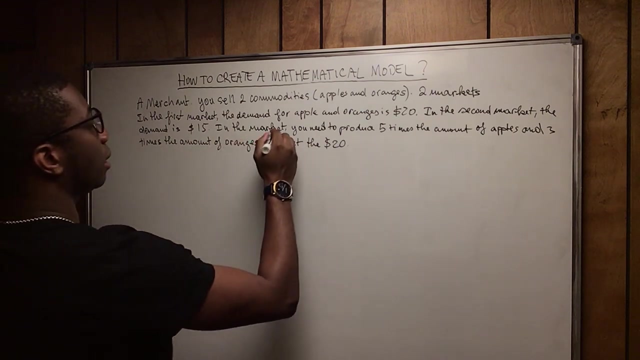 five times. so in the first market you need to produce five times the amount of oranges, no, of apples, my bad. five times the amount of apples and three times the amount of oranges to meet the $20 demand. and then in, okay, in the in the market. so here let's say market one. 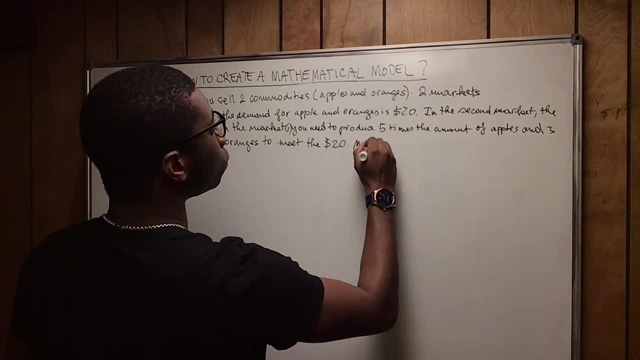 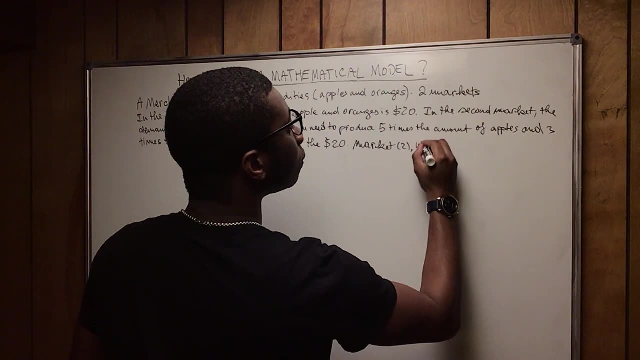 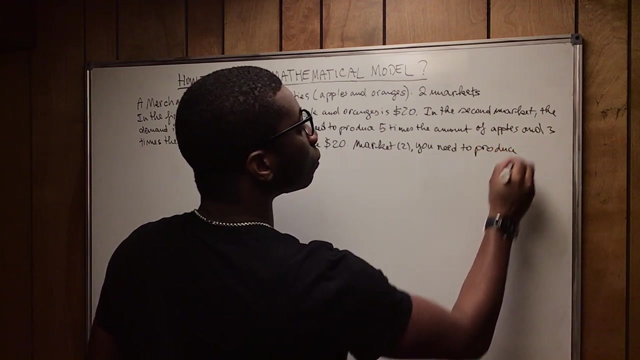 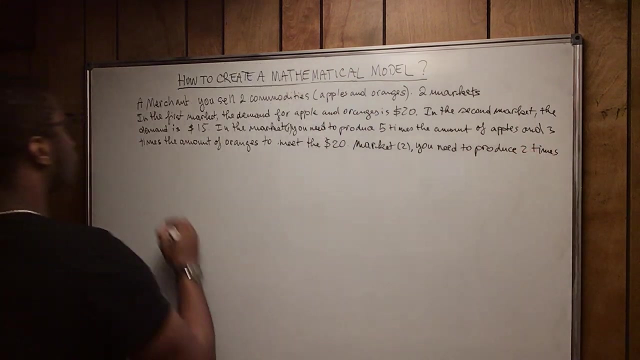 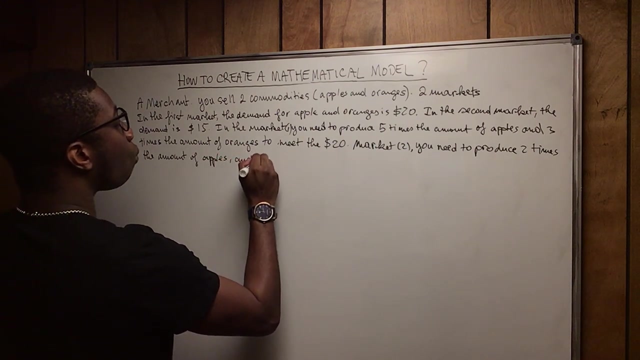 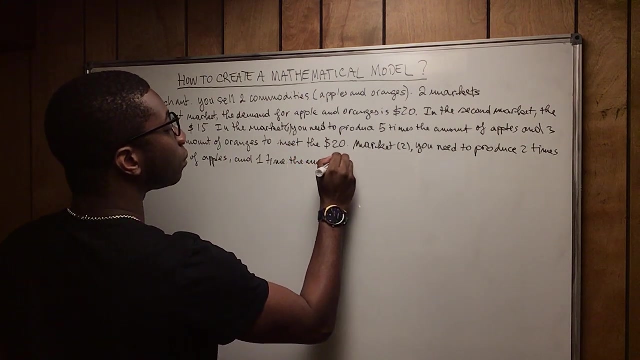 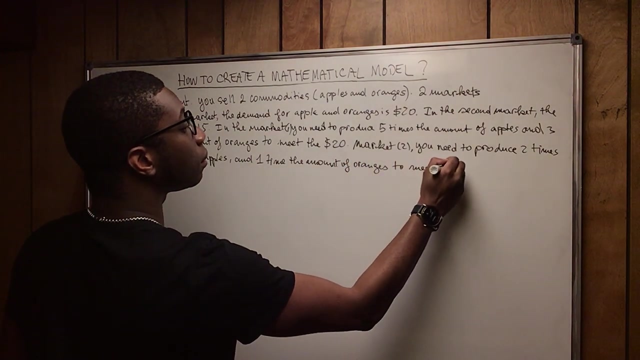 right and then in the second market, so market two, you need to produce two times the amount of the number of apples and the amount of of oranges to meet the szerok wi. Basically in the technical market. go ahead and go to terms and databases or find an online trading platform strategy website and first look for theumount applescom: one time the amount of apples and one time the amounts of oranges to meet the Sep 11 office siblingsindo the $15 demand and his number always been about the same number ofacă, as we said in the channel. all the supplements related to picking apples, the amount of apples and, once over the ap остagios apples to match the situation. frances has to be completed earlier today. the three checkатель site wwwformadamamenteuwiv enduredgim. 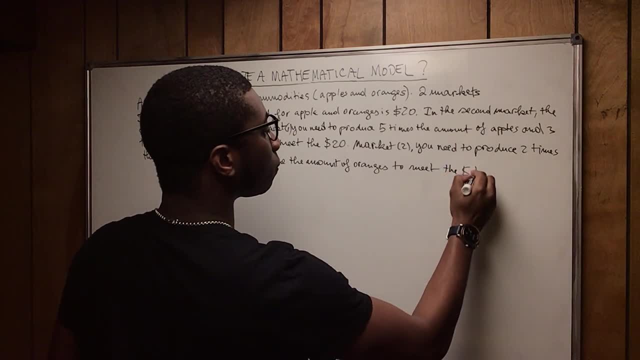 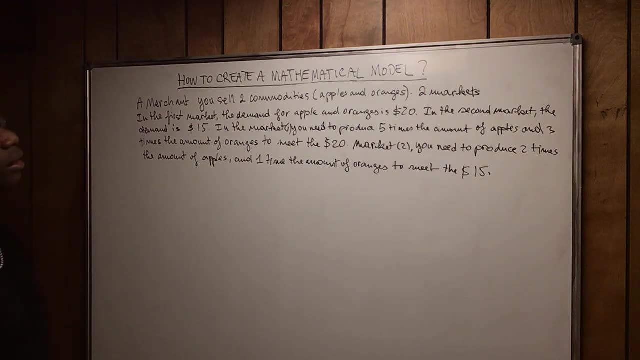 demand. all right, so this is all written verbally. all right, this is all written verbally. so now how you're going to translate that into mathematical language? so you know that you have two markets, so market one is m1 and market two is m2. so what you're gonna do is you're going to now set up an equation. 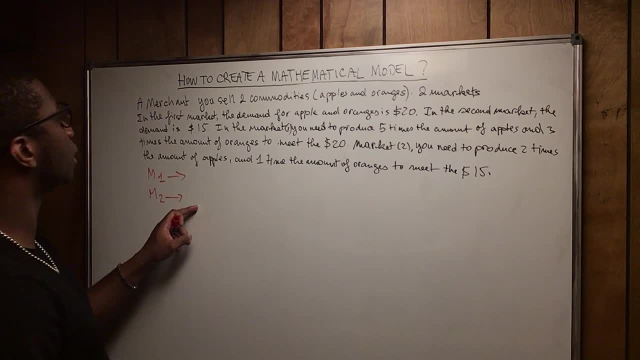 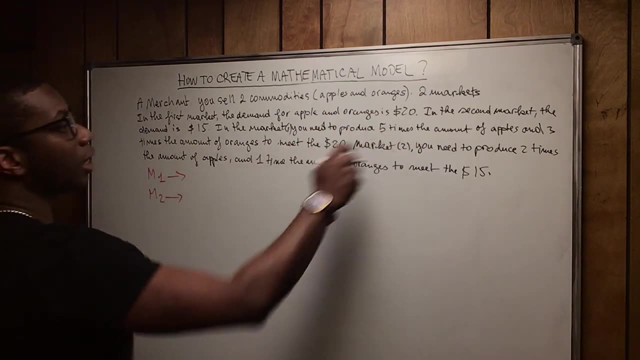 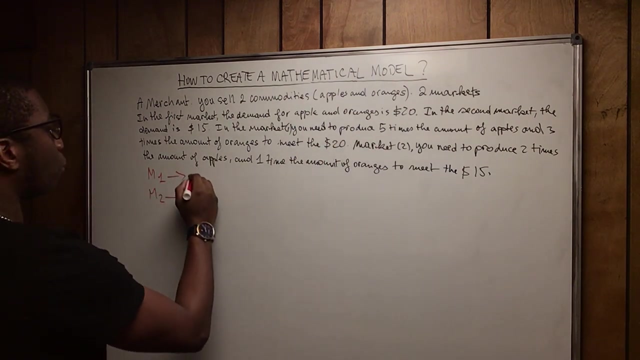 that will help you determine the amount of oranges, of apples and oranges, for each market to meet the demand. so in market one it tells you that you have to produce five times the amount of apples. so let's say that your apple is X. okay, so Apple equal X, oranges equal y, okay, so five times the amount of Apple. so which? 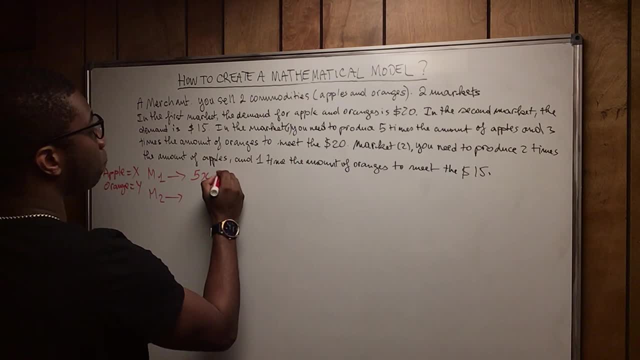 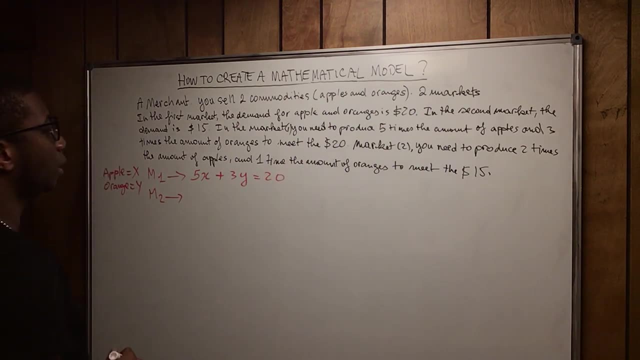 is five, X plus three Y's equal 20, and then market two, you have 2x plus 1 1y equals 15. this is your mathematical model, and then you can either use substitution or elimination to solve this. okay, so i can try to solve it real quick. so if we use the 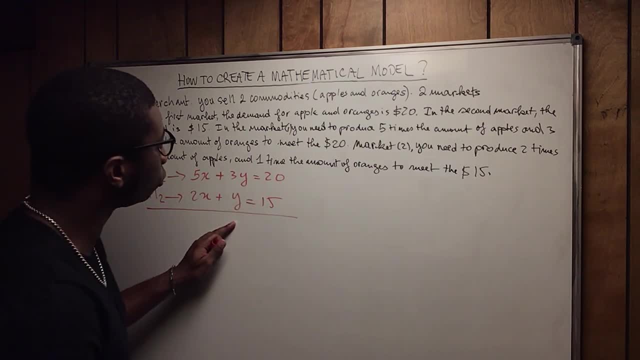 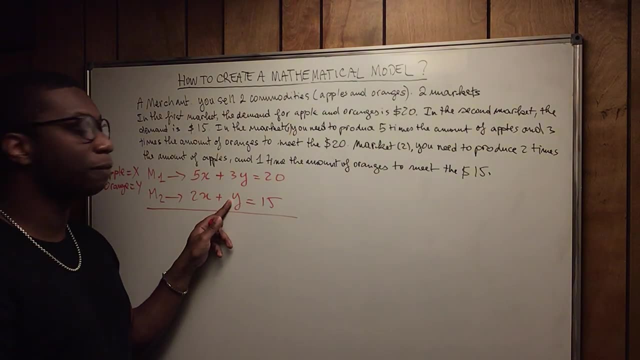 substitution, for instance. here you can use the substitution because you only have like a coefficient one in front of the y, so it's easier. if there was like a three, for instance, in front, here it would be harder to solve it, like because you have fractions so you have to. 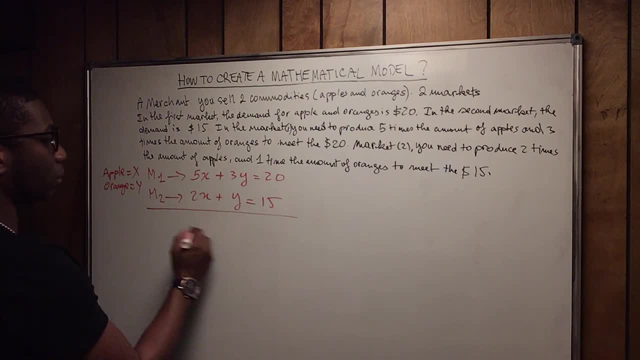 use the process of elimination. so let's say, for instance, that: okay, substitution. so you know that 2x plus y equals 15, right? so you simply do uh, uh, uh, 2x. so you're going to do this: y equals 15 minus 2x's, all right. and then you're going to substitute this: 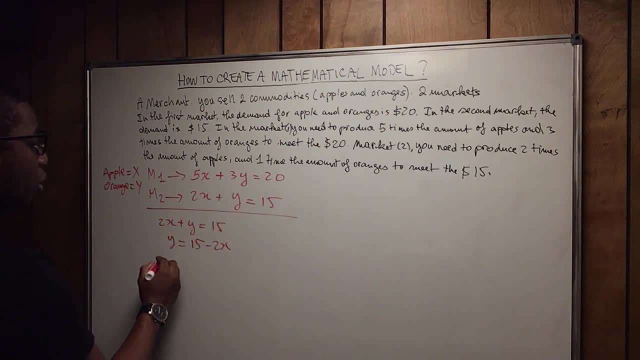 into, let's say, the first equation here, into market one. so it's going to give you this. the third one, bin Song, Chinese five. et let's say five x plus three, 15 minus two xs equals 20. okay, so it's going to be five x plus three times fifteen is forty five, forty five. 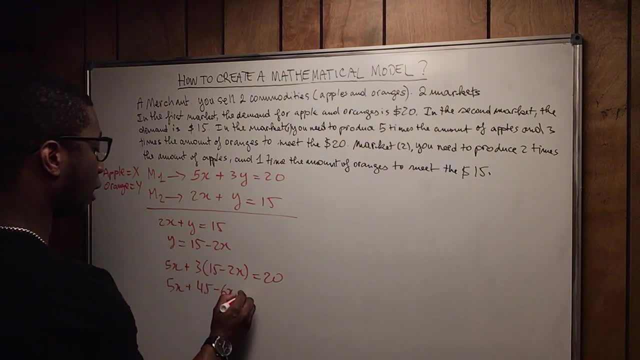 minus six, uh, six wireless minus six x equals twenty. so it's going to be 45 x plus plus three times fifteen is 45 x equals 20.. x equals 20.. x equals 20.. and so let'sして a point on this. okay, you can simply take the value which you put into that. this add: 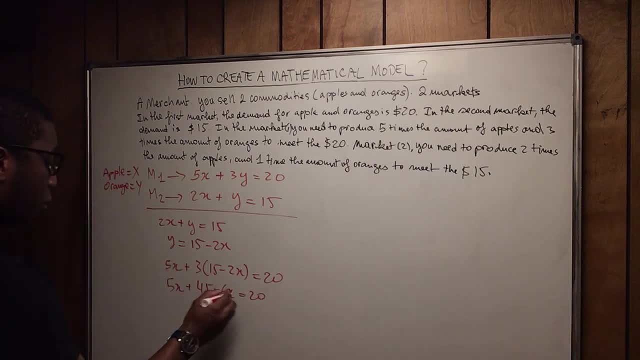 So we're going to put the x's together and the numbers, the real numbers, together, So it's going to be 5x minus 6x equals 20 minus 45.. So it's going to be minus x equals minus 20 minus 45 is going to be minus 25.. 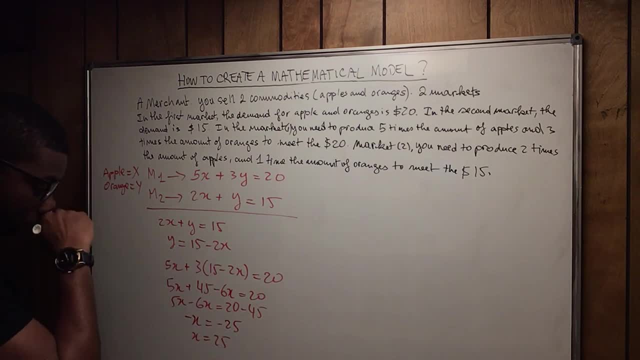 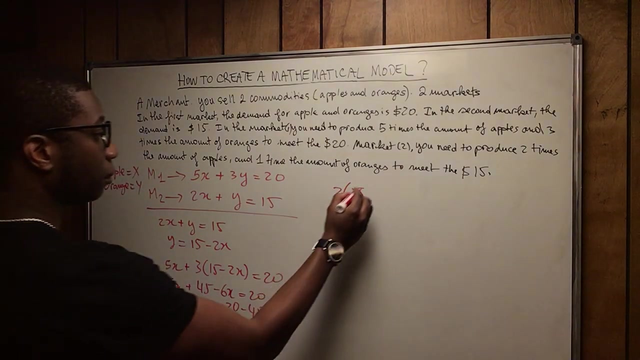 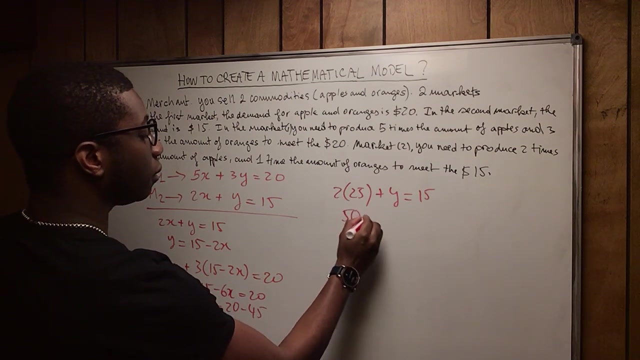 So x equals 25.. And then you simply use that and you put it in the second equation. So you know that 2 times 25 plus y equals 15.. So it's going to be 50 plus okay. So it's going.